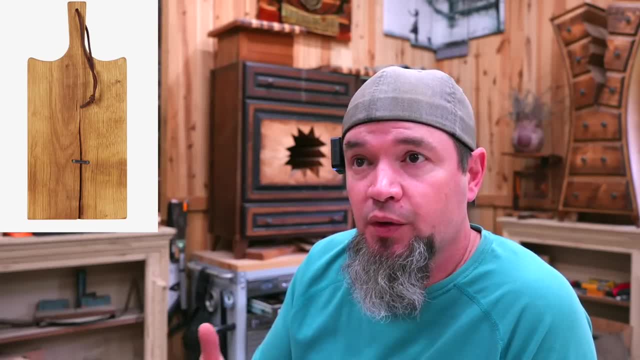 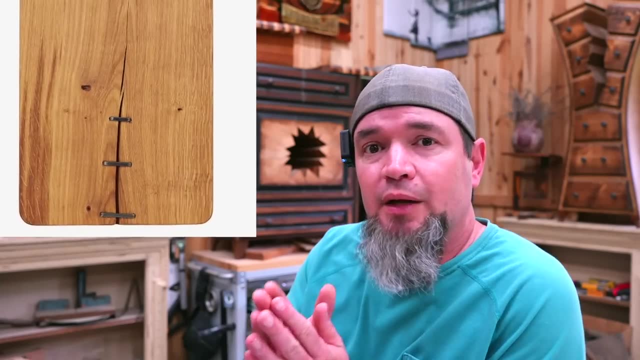 would bust a table, bust a piece of wood, if you could not cut dovetails and put those in. you did this: You would bend over a nail or a piece of metal, whatever that you had, drive it into both edges of the split and it would keep it from splitting more. 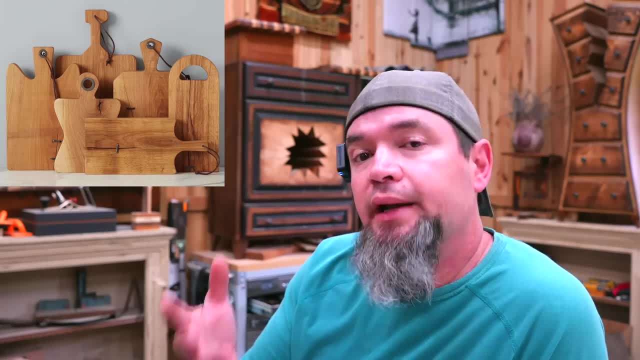 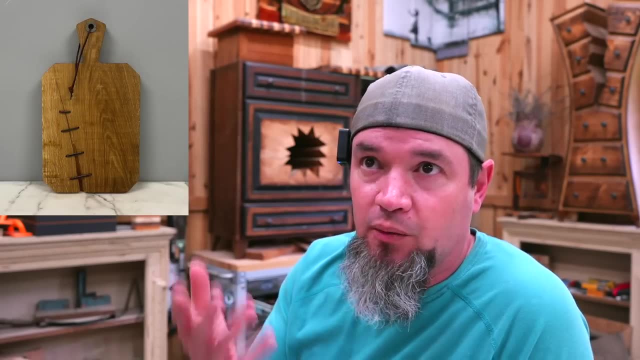 Seen this done before on super old farmhouse tables, but never on a cutting board. I'm just going to call it a cutting board from here on, because I don't like saying decorative paddle. I mean, it sounds like you're about to whip somebody with it, So really the only 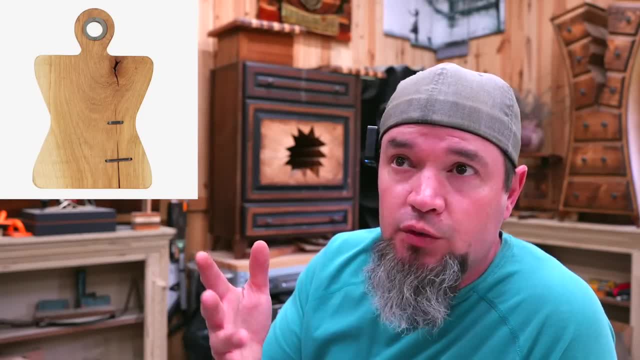 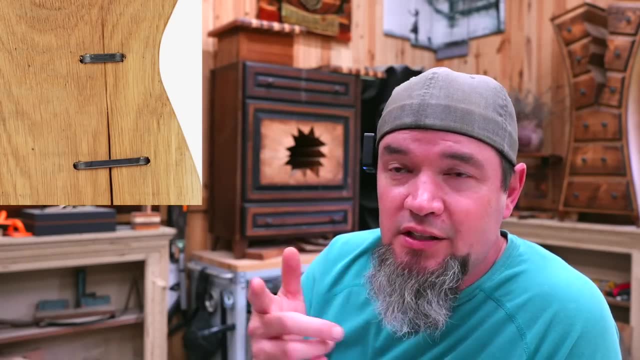 difference in this and other cutting boards or charcuterie boards or whatever that you want to call it- that we've covered in the past, is that split in This is awesome, because oftentimes, when we're working with wood, these are the pieces that we're just going to toss that are naturally split. 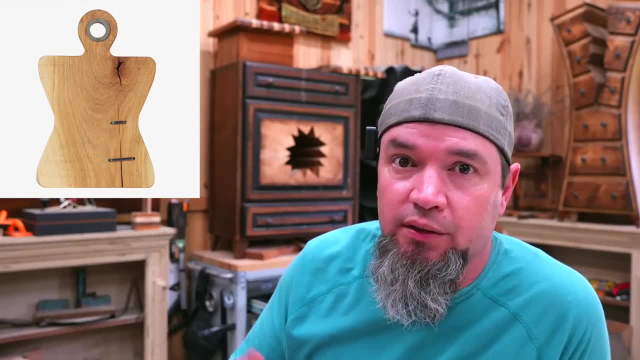 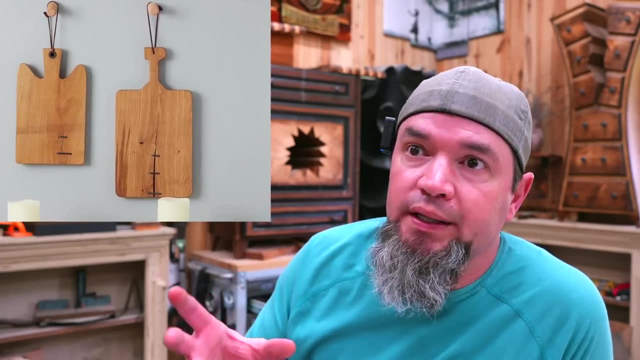 So, as far as the outline and the design of these things, you already know how to do it. There's a out there and we've actually covered it ourselves. It's super easy, especially on these one plank boards. So if you're wanting to replicate this, of course you have to have an end cut with a crack. 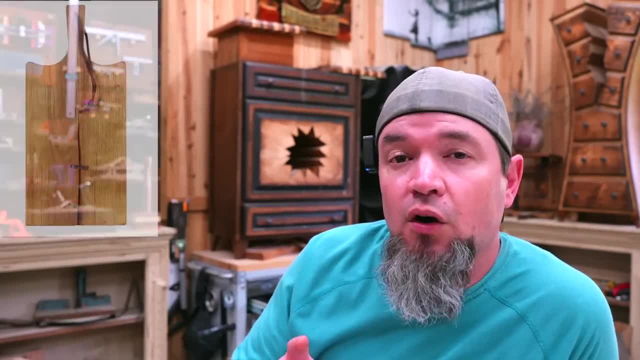 in it. Well, we're not going to have a ton of those, so you can make your own. That's all that you'd have to do is take your plank of wood, maybe put one end in a vice and just start bending it a. 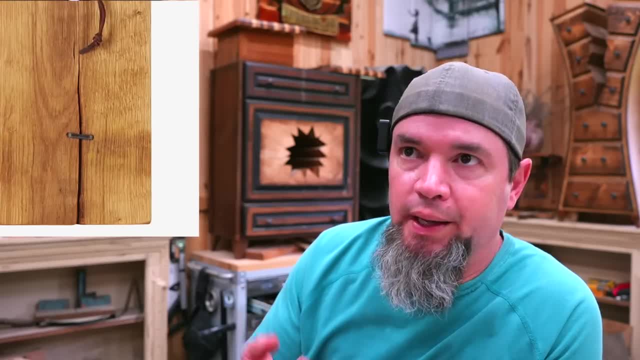 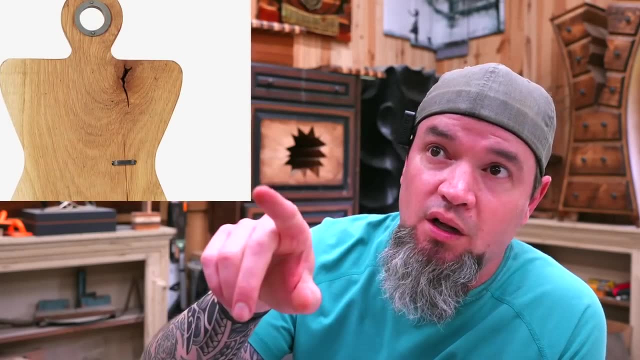 little bit. Be careful, Do not bend it too fast or it will snap all the way. Let's say that if you're using something like pine and that the pine's grain goes all the way up, it's going to split completely in half. If you notice, on a lot of these there's a swirl. 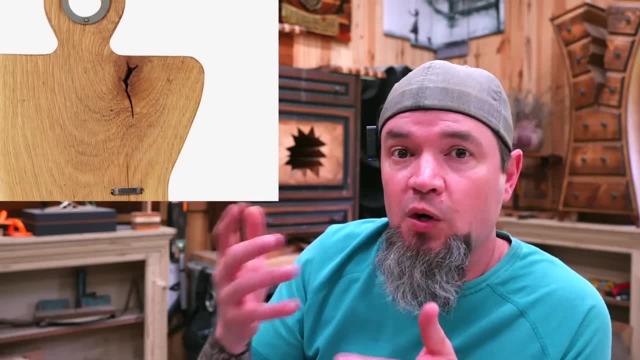 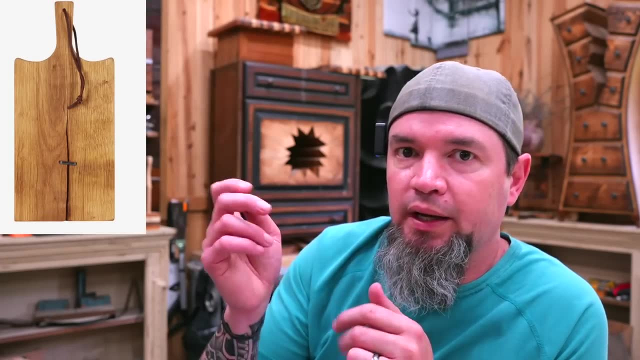 in the grain. That's what's going to help stop that crack from going up. Or, if you notice, in a lot of these it's a fibrous type of wood, like this oak, So it's not just going to snap. Those fibers are going to want to help to hold that together. So if you're creating your own crack, 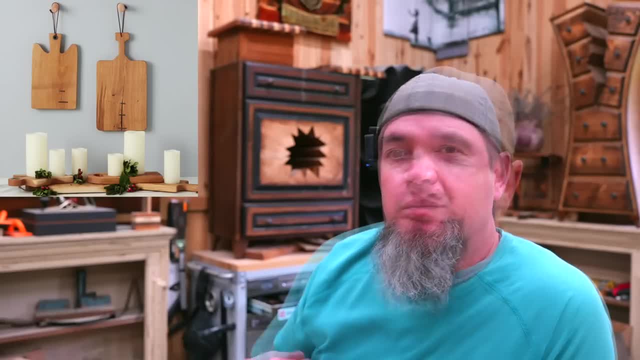 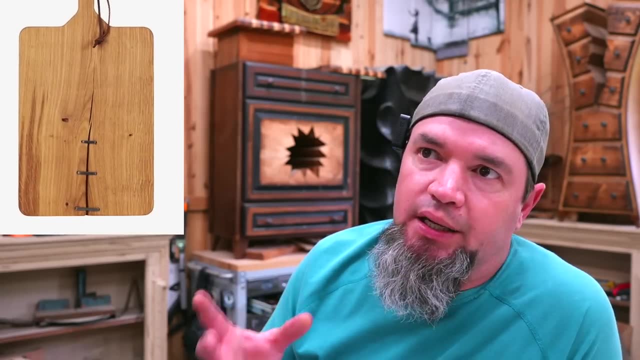 maybe try to use a wood that's kind of similar to that. So once you have your crack material- be it a scrap piece of wood or something that you have put the crack in- now we need to create this stitched look And it looks like what they have actually done is they've used some type of a thin. 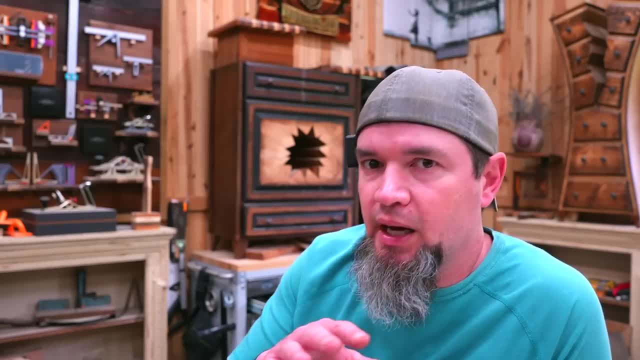 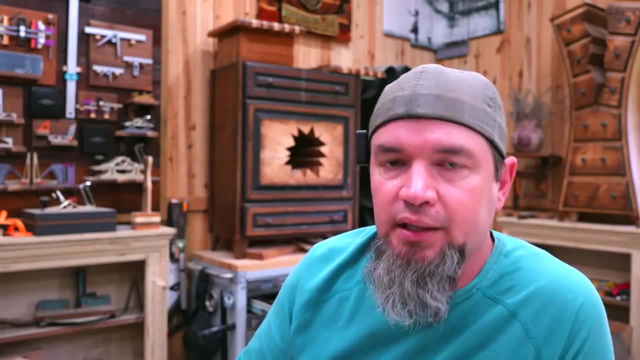 square stock. Post this thing that I could think of. Now, help me out here. You guys can think of anything that's kind of thin and square. Drop it into the comments, because I was drawing a blank on that. What they used to do back in the old days, they would take a square nail. You still? 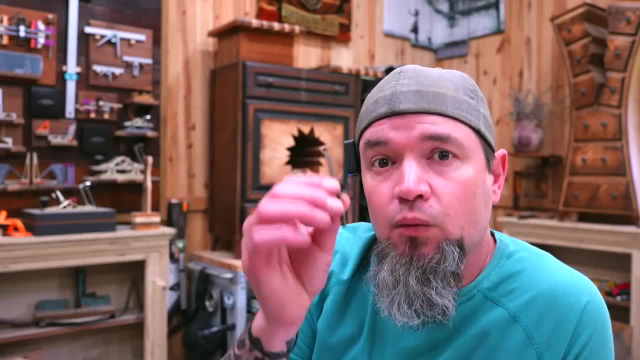 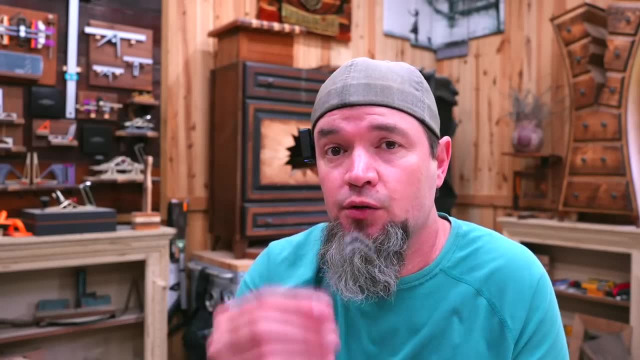 buy these square nails. They may be listed under horseshoe nails, But what they would do is they would take these and they would actually bend these to make a staple. So, whatever you decide to use, you can use this. You can actually use a new steel nail. See where I just bent that end. 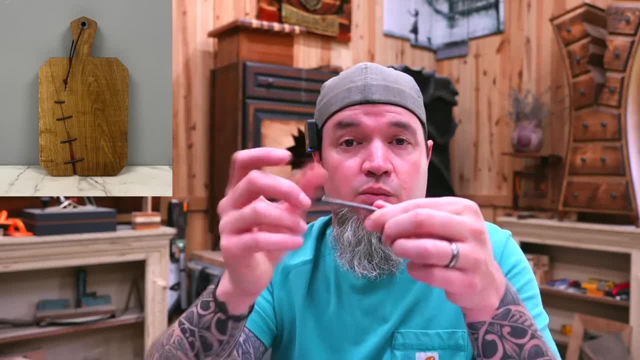 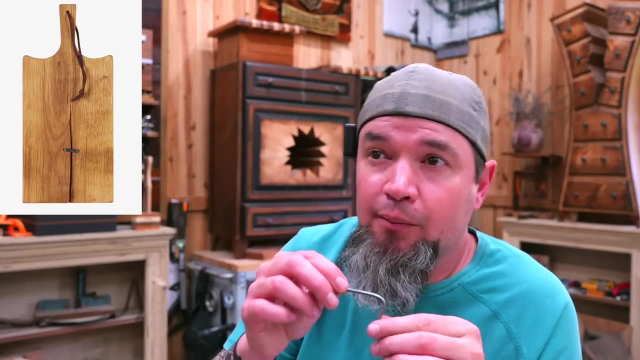 Depending on where you're at on the gap. put this in a vise, pair of channel locks, whatever. Then you just bend this down, snip off the end to make a staple, Paint it black. No big deal and super cheap. Instead of hammering this in, go ahead and pre-drill a hole on both sides of that crack. 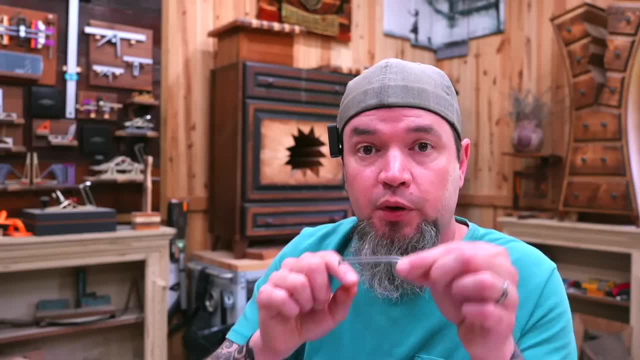 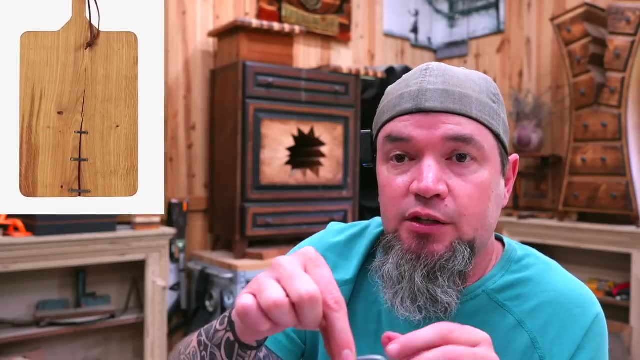 that is the same distance as your staple that you have made. Put it on your board, mark it. drill a hole on each side of that crack, Put in a little bit of epoxy adhesive on both sides and just slide this right in. Let that dry. You're good to go. Finish this out, Really. 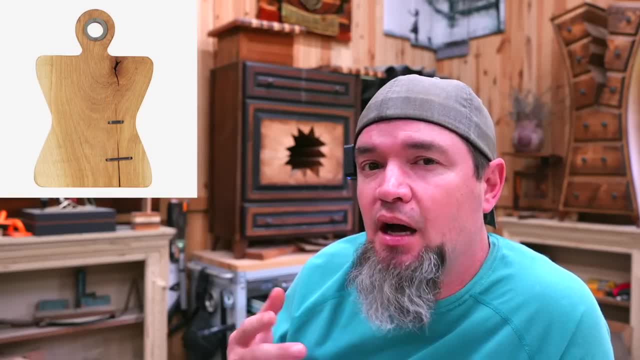 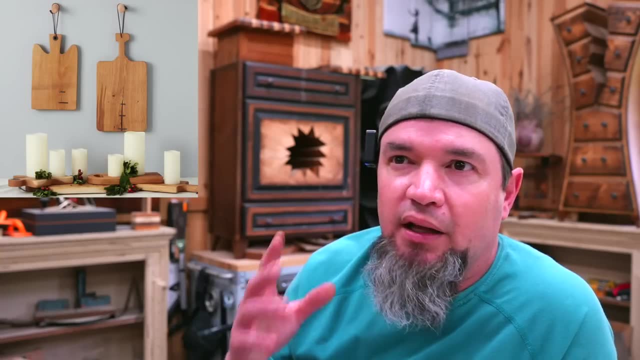 you can finish it out in any way that you would like, Since this is technically not considered a cutting board. it's a paddle and it's really mainly for decoration or for a serving tray. Most likely, they just applied like a clear polyurethane finish on this, But if you'd like, 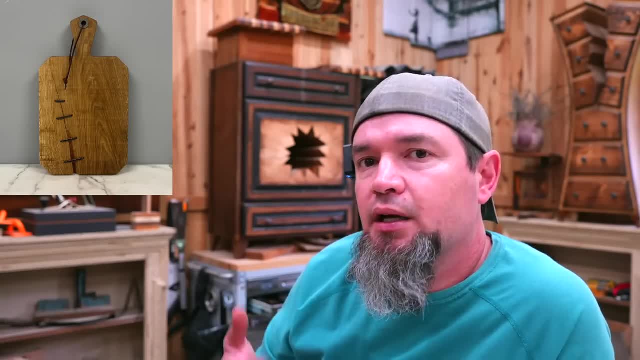 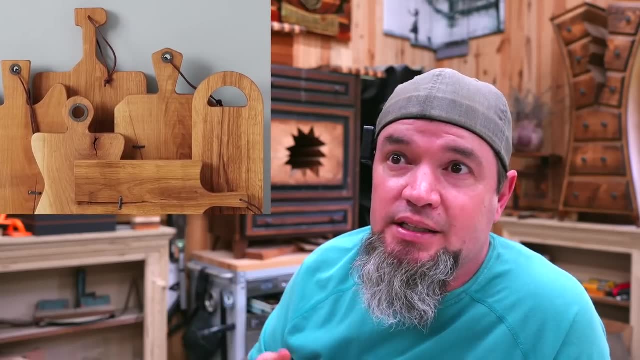 to make it to where people can cut or eat off of. then you'd use like a cutting board or something like that. Either way, super easy to make And the handles any shape that you want. As you can see, they just kind of cut whatever shapes that they would like. You can do the same And for the tops. 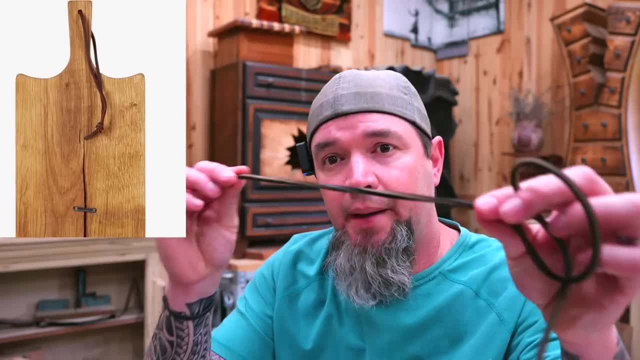 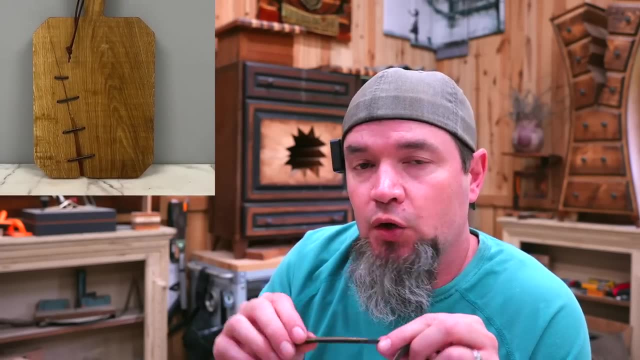 that's. all that they have done is drilled a hole and put a leather strap in there. You can pick this stuff up. They're super cheap off of any craft Or off of Amazon And after I thought about it, as far as the crack goes, you could actually use. 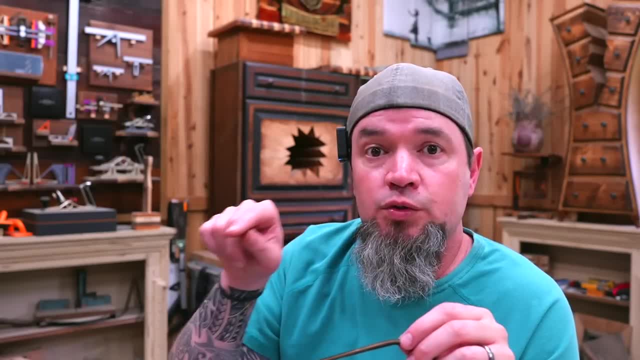 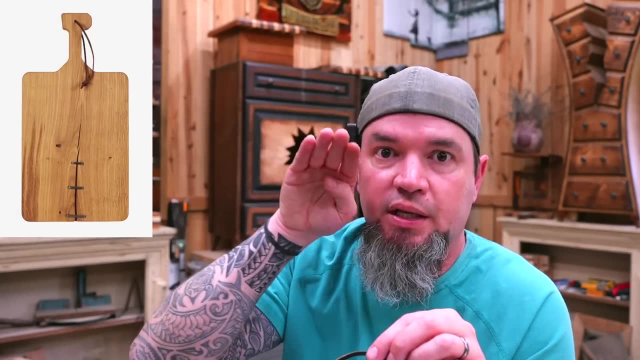 this leather strapping instead of any kind of a metal. Drill your holes all the way through. Then you could run your stitching design all the way down And depending on the pattern that you want. if you want this pattern where it's just the flat bar look, then you would just feed it in. 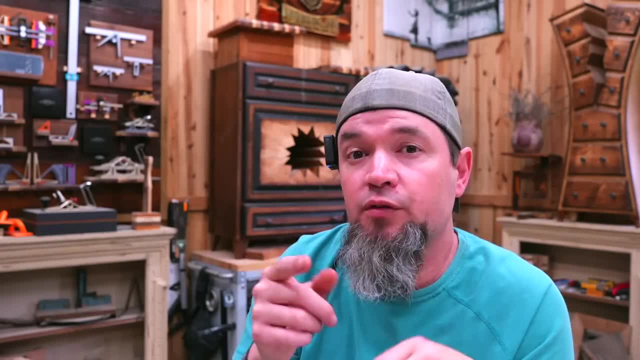 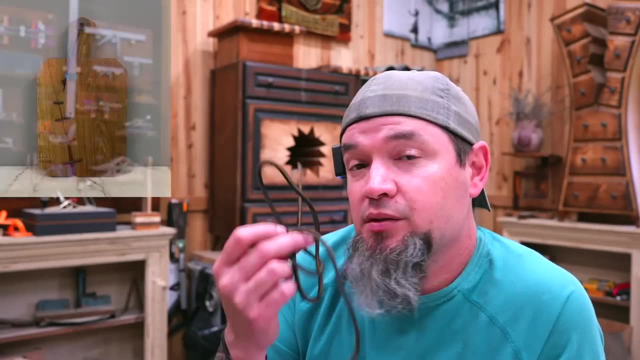 and put your cross section in the back, go down back over. Or if you actually wanted the stitched look where it crosses, then you would just thread these through in the opposite way. Then you would run that pattern on the top. So that was just a quick idea. 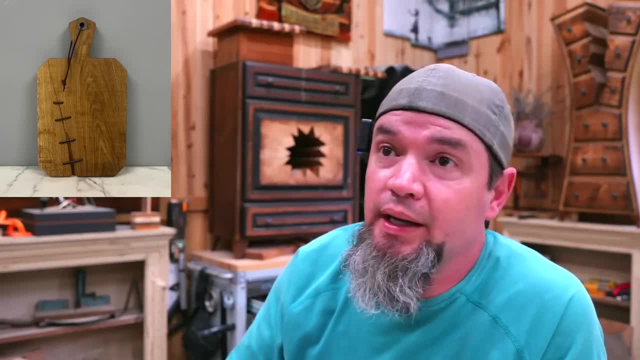 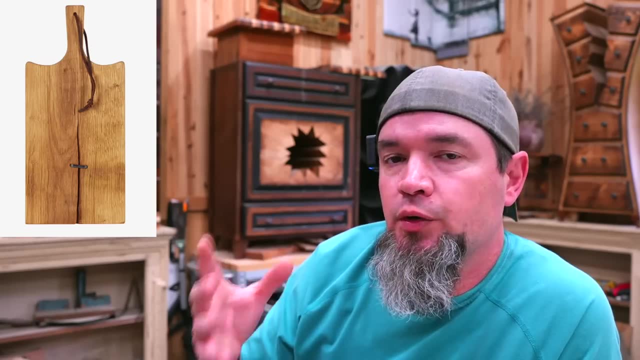 I think that I like the leather idea better than that one. Either way, it's a super cool product. The old PB is wanting $80 per paddle And they've created different size paddles because people will buy two or three to set around their house. So $80 a piece. If it were me, I would try to move. 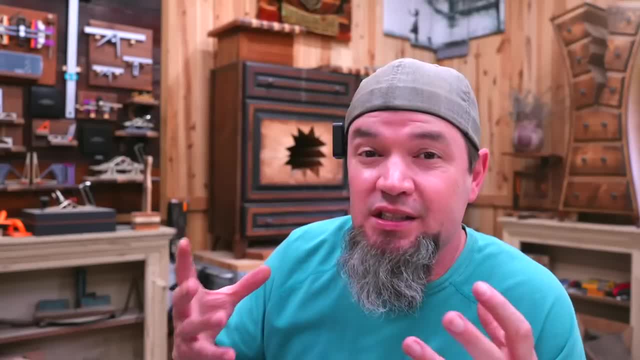 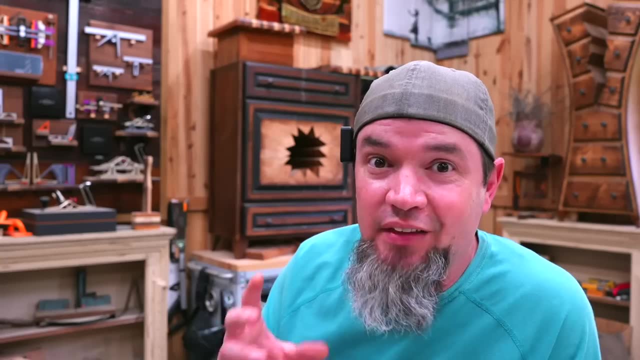 these in the $30, $40 range and sell them as sets. So this is another one from the PB, And I had to throw this one in here, since we're already talking about this decorative paddle serving tray, whatever they want to call it. Now they have also came up with this style. Okay, so they're calling. 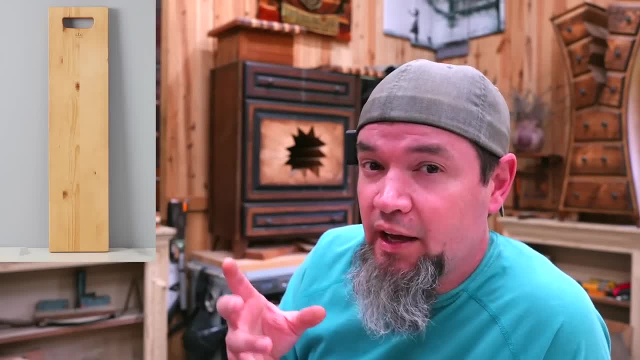 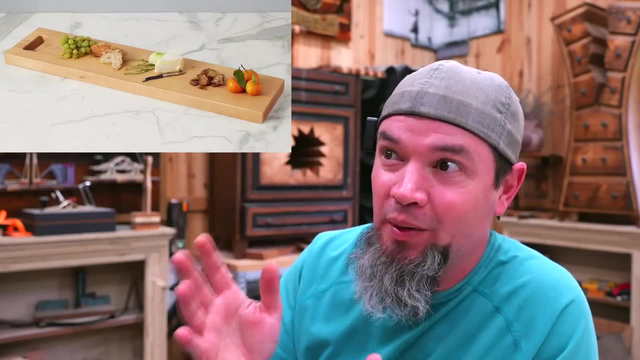 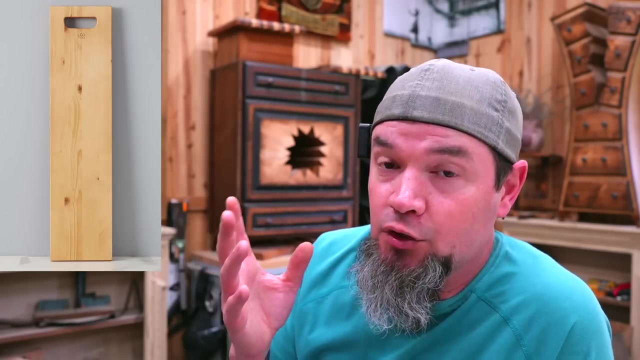 this a modern cheese board, because the dimensions are one and a half by seven and a half by 26 inches long. That is a two by eight. Look at it, It's just a square two by eight. It's either pine or fir, but it is a two by eight. So for $130, they are selling a 26 inch piece of a two by eight. 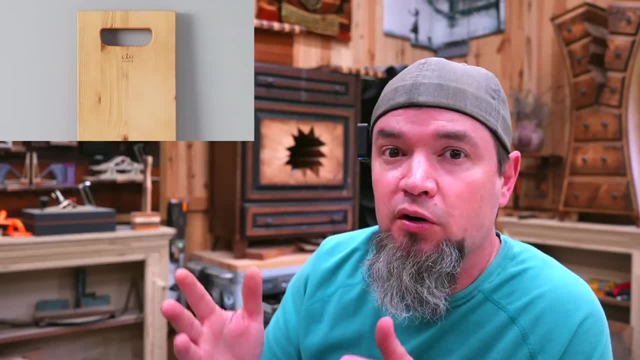 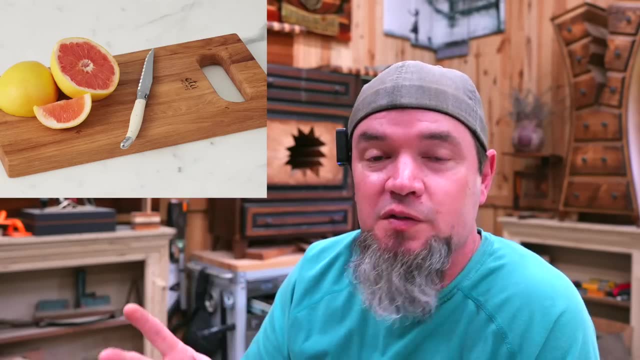 with a hole cut in the end, And they're calling it a modern cheese tray, Calling it modern just because all of the edges are perfectly square. We don't have the contours, We don't have the curves, We don't have all of that, It's just square, Even the handle, that's. 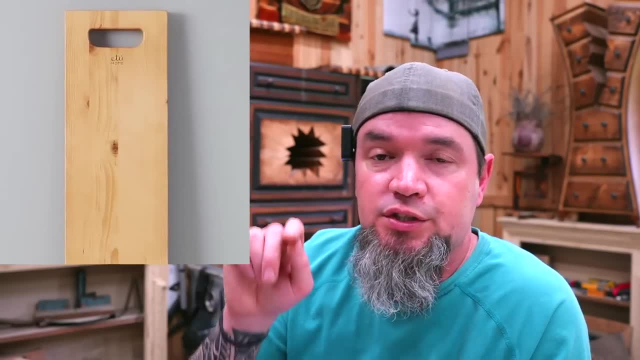 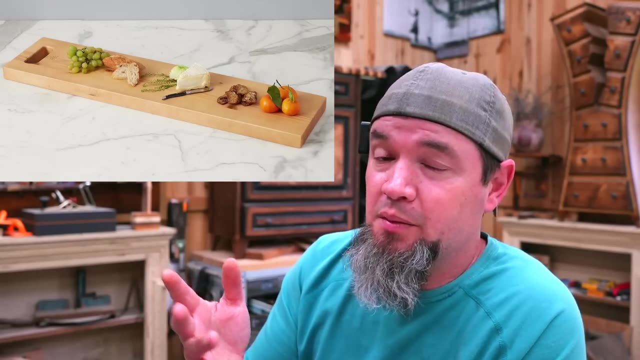 cut into it is more of a square shape instead of the rounded shape. I'm not going to spend any more time on this, I just had to throw this in there. This is pretty self-explanatory on how you do this. You finish it with some type of a board oil. I do not know how well these things 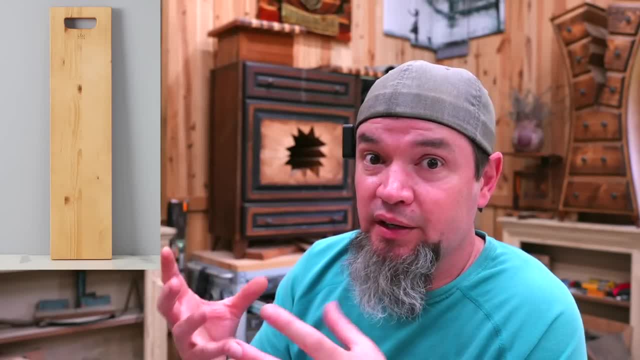 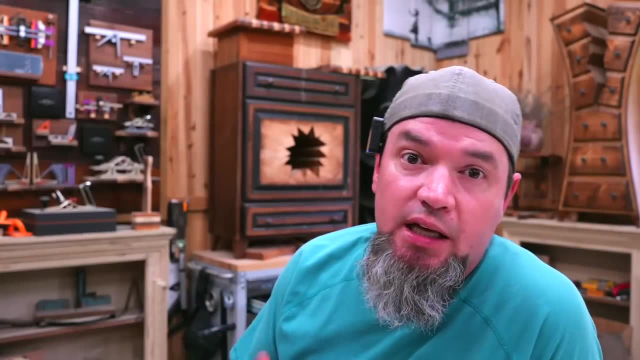 would sell. I know that they are selling them, or it would not be on their site or in their stores. But like I teach, just because I don't like it doesn't mean that someone else wouldn't like it. So give it a shot. And this next one, a wooden star. 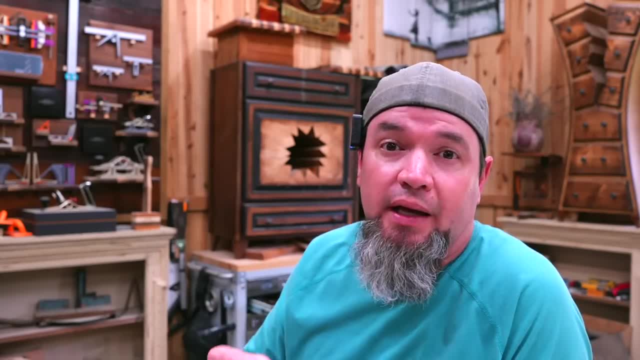 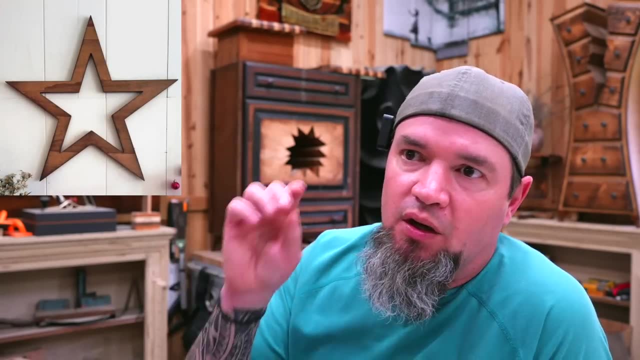 I've talked about these types of items in the past that have always been popular and pretty much always will be- The nautical themed items, star items, hearts, things like that. But what got my attention on this one is it was listed as a best seller. It is completely made out of. 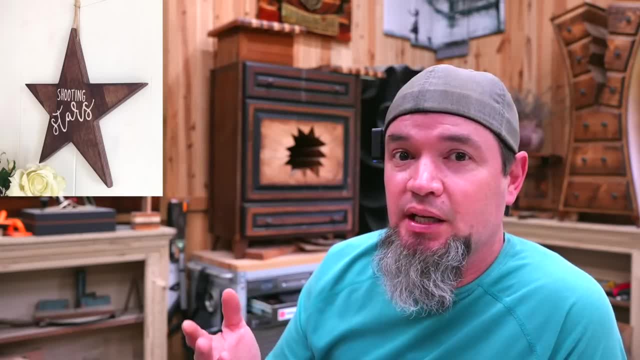 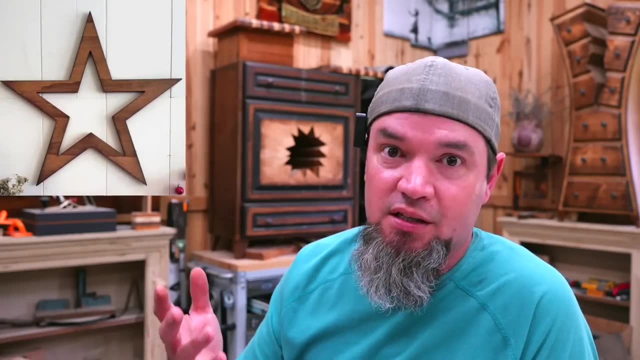 plywood and they are wanting 68 bucks for this thing. Yes, it's three quarter inch plywood and three quarter inch plywood is expensive. But this doesn't even look like cabinet grade plywood, It just looks like plywood. But regardless, this is a 24 by 24 star. 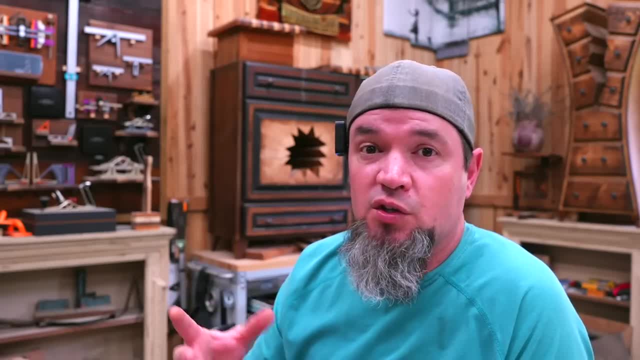 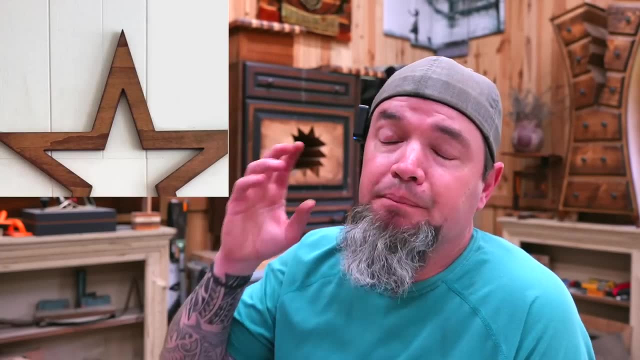 In a previous video I actually taught you guys on how to draw a perfect star of any size. But if you're interested in something like this and you don't know how to draw a star, you can check that out. But the cool thing about this is that it can be completely cut out just. 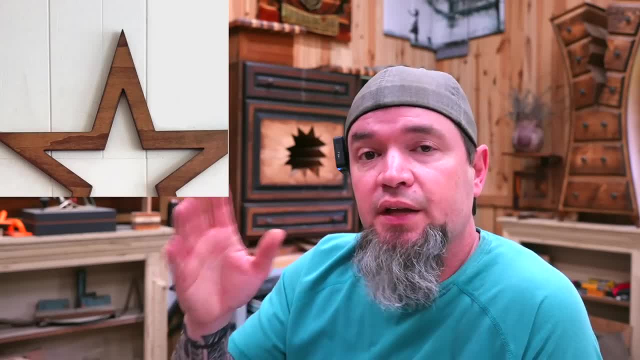 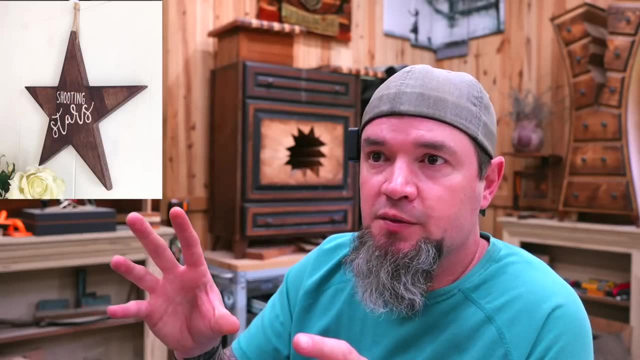 using a jigsaw, regardless of whether you want to make the version where they have cut the center out as well, making this negative space star, which is pretty cool, Or if you just want to make the solid version with no negative space and put some type of writing or saying on that. So let's. 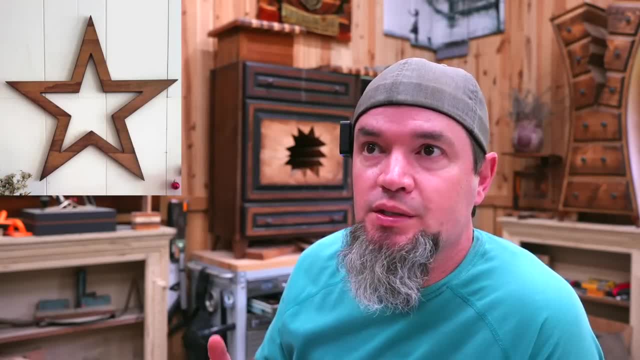 say that you wanted to make this star with a negative space And the only thing that you have to use is a jigsaw: You're really going to want to make this star with a negative space. You're really not going to be able to save the cut out from the middle, which would be super awesome- because you 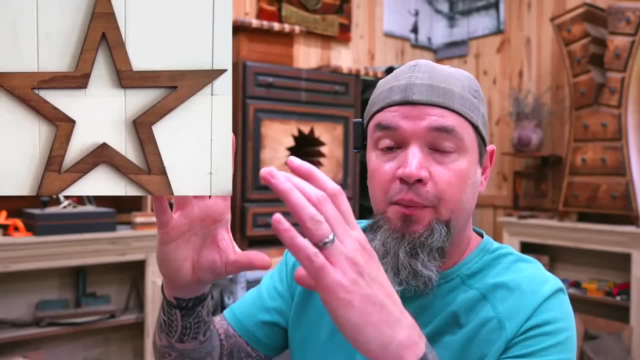 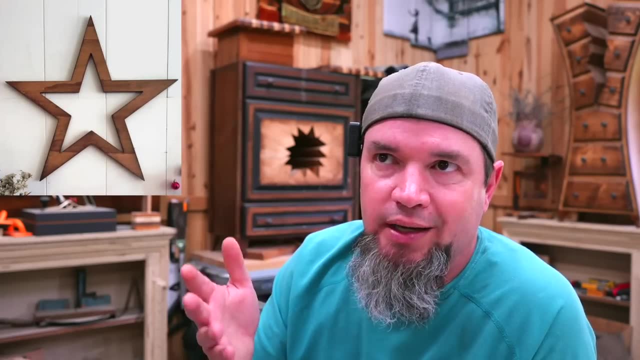 would actually have two products to sell. You can sell the main outline and then the part that you cut out. There is a method that you could use with a jigsaw where you actually walk the blade into the wood, But I'm afraid with plywood it may create too much of a tear out. If you have a 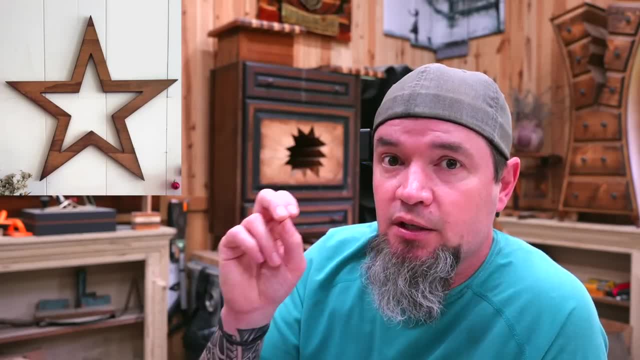 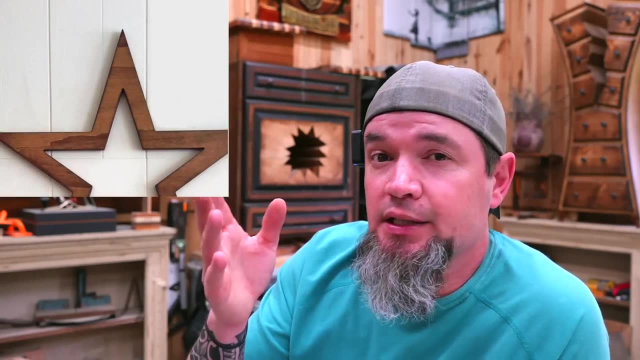 router. you could, however, cut this out with a router and be able to keep that center part. Or if you had an oscillating tool with a wood bit on it, you could cut this out with that as well. But regardless of whether you keep the center or not, the next thing that you would do for this 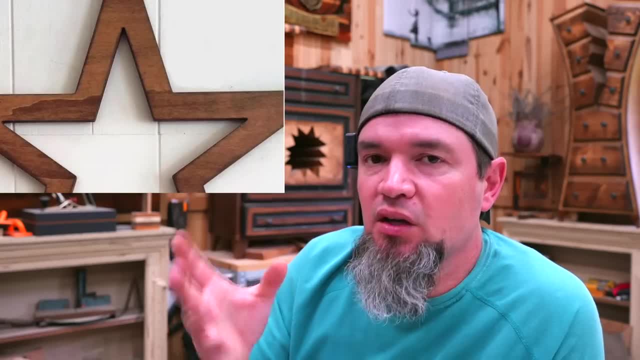 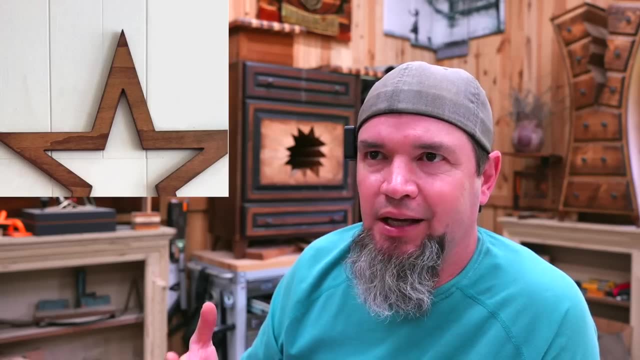 star is to stain or paint it And in the end, you're going to want to make sure that you're and it actually looks like they want people to see that it's plywood. I don't even know what kind of a look that you would call that. I don't know if it would be like a modern industrial or. 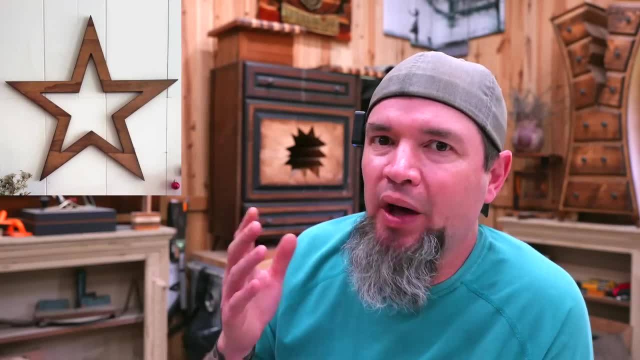 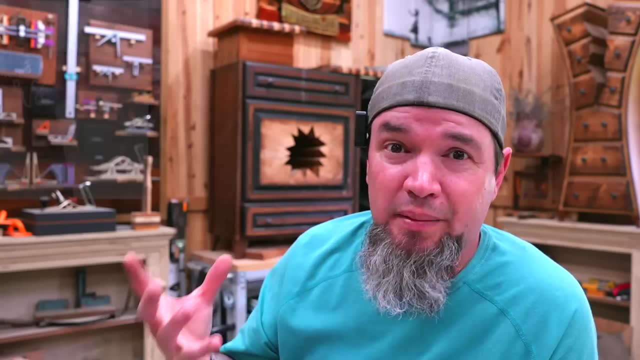 whatever, but they're making zero attempt to hide that it's plywood. You actually look at the edges of this. You can see where all the different layers are glued up, which is obviously plywood. So maybe this is the end thing. If it is, let me know, because I have no clue. So these are 24 by. 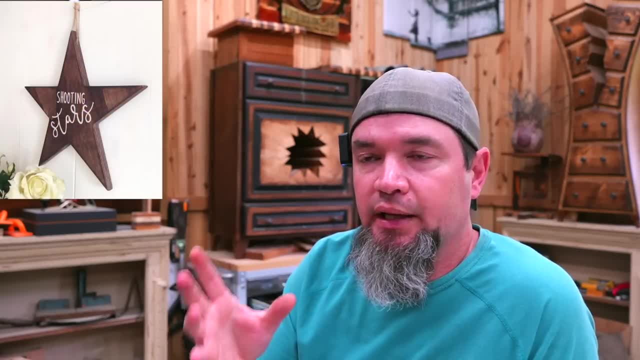 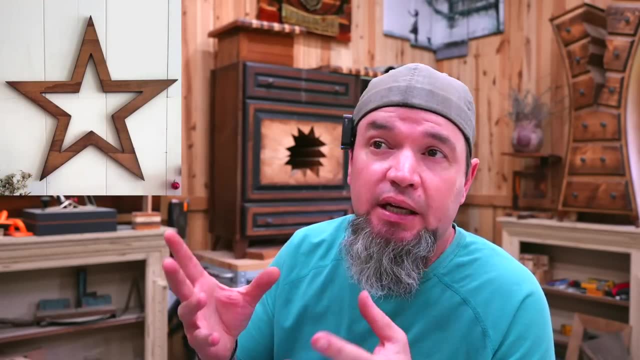 24. So they're very large stars And that's why these things are selling. So if you use those dimensions and you just start with two by two squares and get eight of these out of a sheet of plywood, they're wanting almost $70 for each one of these. If it were me and they were stained or painted, I would try to. 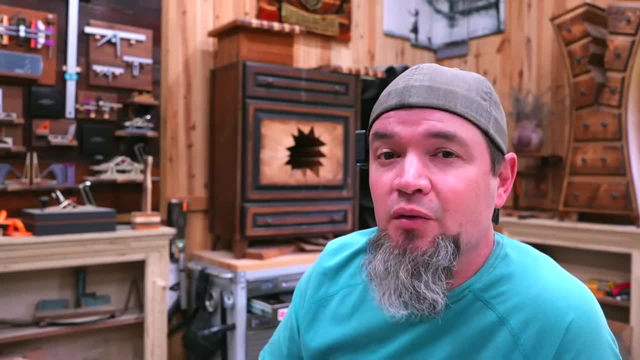 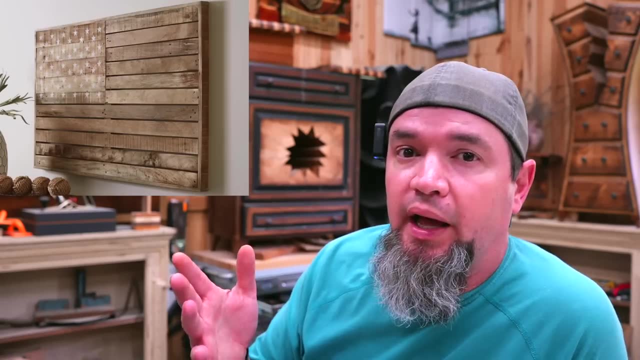 move these right around the $30 mark And that would still leave a ton of room for profit. So this next one I really, really like- and I know that they would sell like crazy- And that is this pallet wood wooden flag. Okay, So I know that there are tons of versions of wooden flags out. 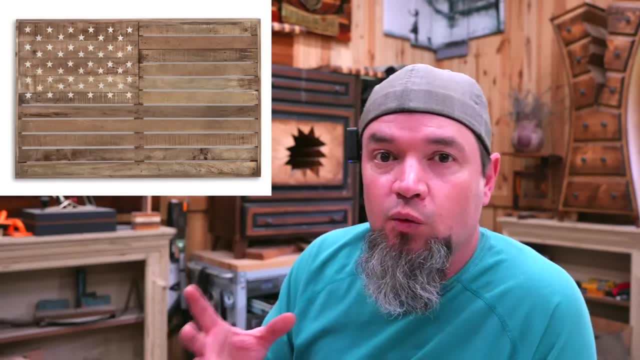 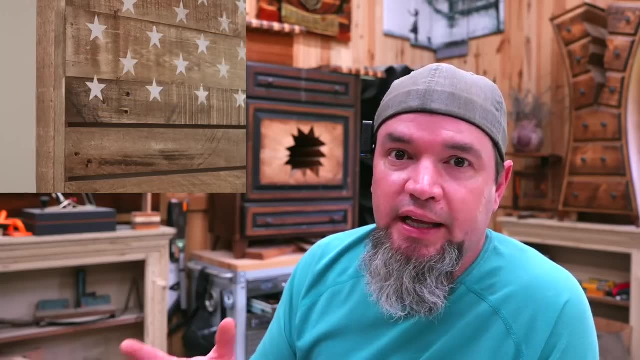 there. but there's just something about this. But this would be your perfect pallet wood project, because pallet wood looks just like this: It already has an L hose, It's kind of beat up and you want to leave all of that in there. You could easily 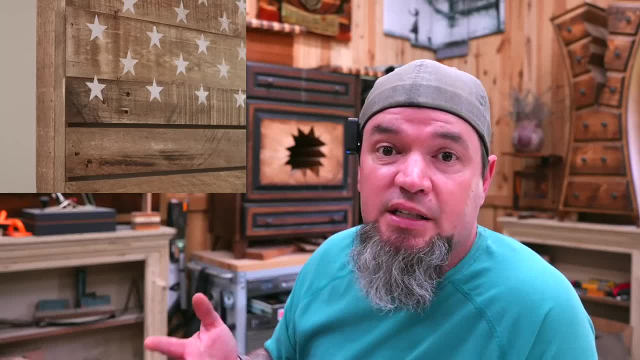 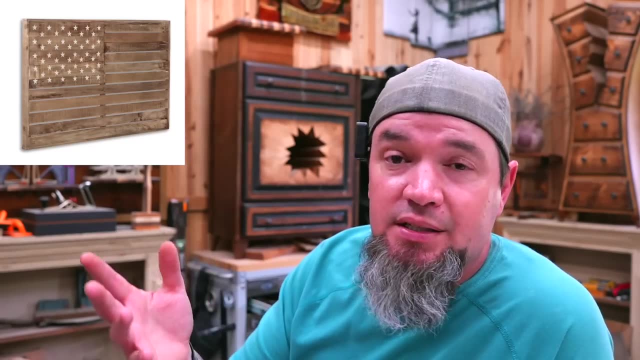 replicate that if you wanted to make this out of fence pickets, But for this one it may just be easier using pallet wood. They are wanting $150 for this flag And honestly I don't think that they're too far off. If I were making these to sell, I would probably try to move them right. 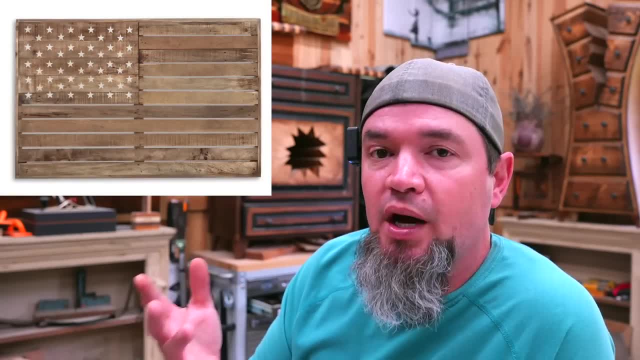 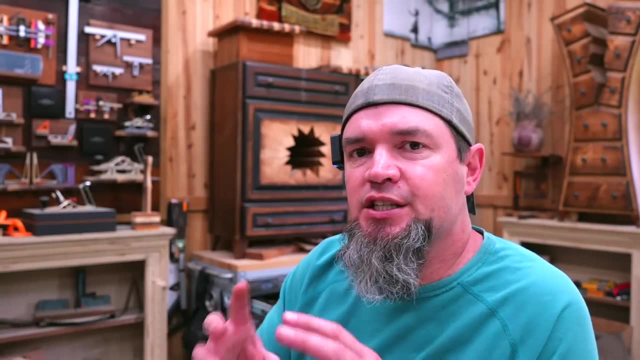 around the hundred dollar price point, And it's because it's different- You do not see these everywhere- And I guess one of the reasons why I really like this look, but because it reminds me of the inside of an old house that had, like the ship lap and the plaster. Okay, So if you've ever 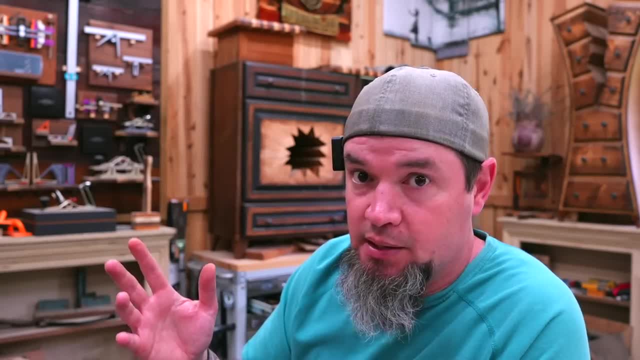 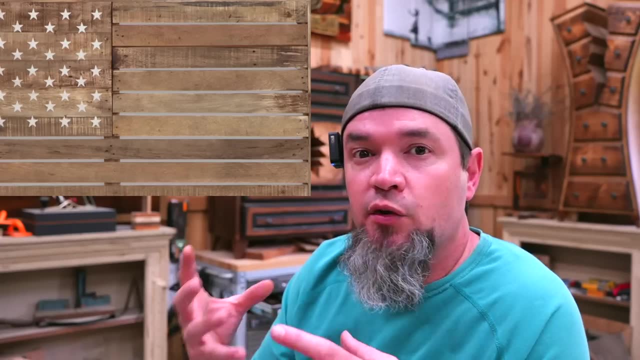 seen behind one of those walls or if you've taken off all the plaster. it's a big mess, but if you've ever done it, you know what I'm talking about. It's just those thin strips about two inches wide, with about an eighth of an inch gap in between, And it just creates this. 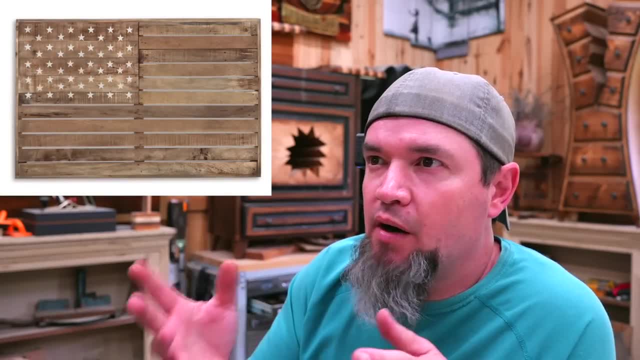 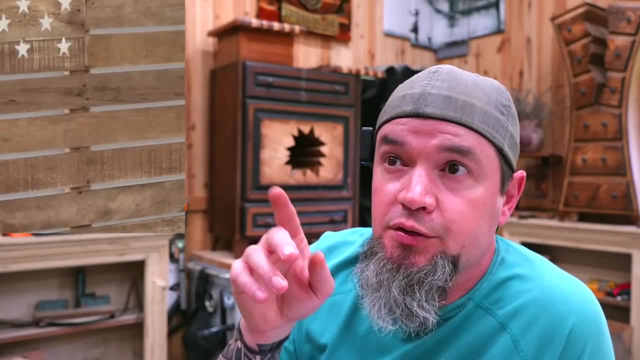 cool vintage look. So let's talk about how they put all of this together. So obviously, you can see that they've used the strips on top, but it also has a border around it. Okay, We're not going to put the border on, yet. If you look through those cracks, you can actually see vertical strips. 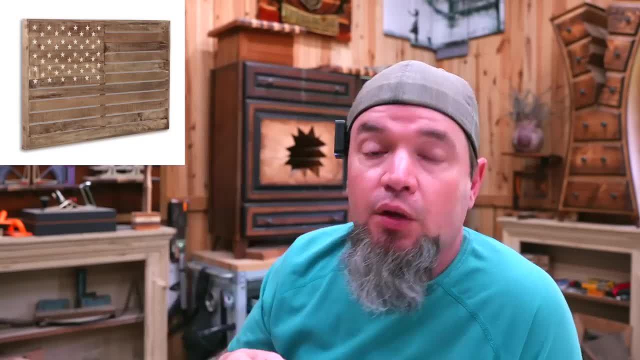 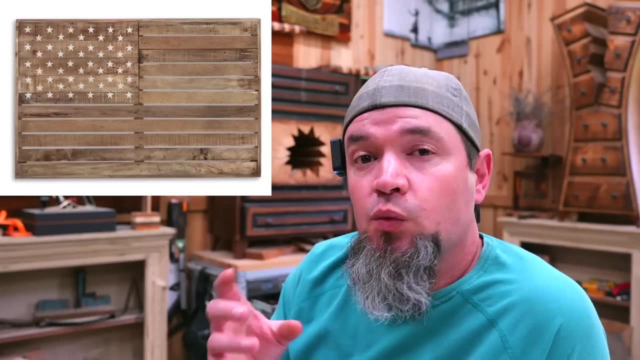 The size that you would like, whatever width that you would like this to be. you can go ahead and cut three strips for the back using the same material that you're going to use for the top, And these strips are just going to be. connecting strips is what is holding all of these strips? 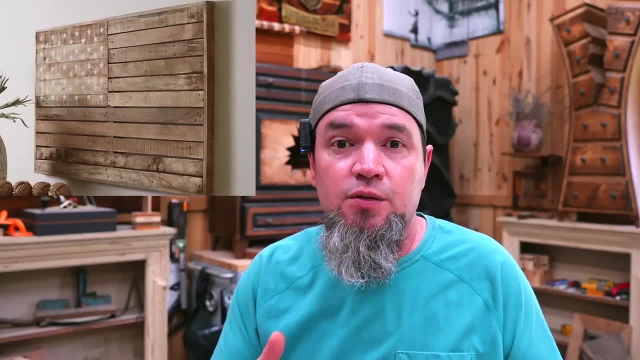 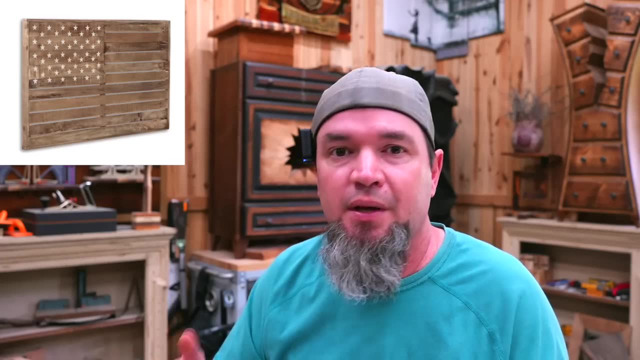 together, So you'll need one on each end and one in the center. Then you were to space those out to the length that you want. So the halfway point is where they ended their section for the stars. So, starting from the bottom, I'd take a 48 inch strip. The thickness of these strips really do. 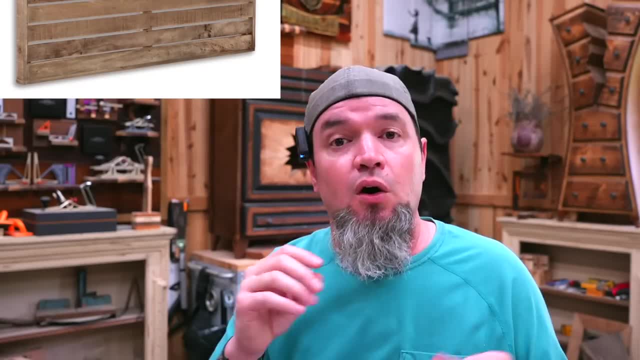 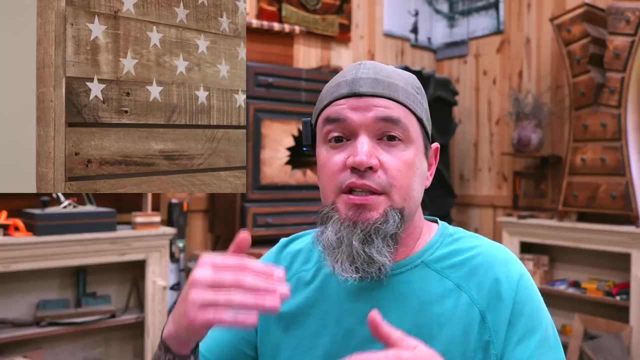 not matter as long as they are the same. Now I would attach it to the bottom to all three of your horizontal boards And really I'm going to take a 48 inch strip and I'm going to take a 24 inch strip And you're just going to cut 24 inch strips to finish the right-hand side And we 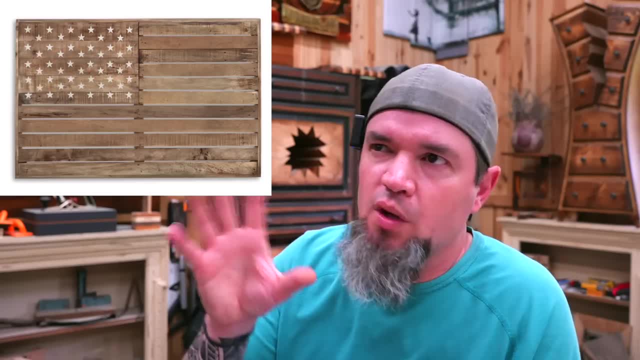 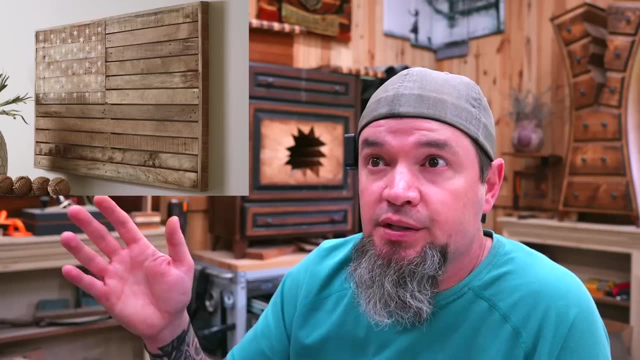 will use the same spacing as you did for the bottom. You want to actually be able to see through this. So now you've attached the complete right hand side as well. Now for the bottom. I'm just going to cut the extra strip for the stars. I'm going to cut it off. So this will 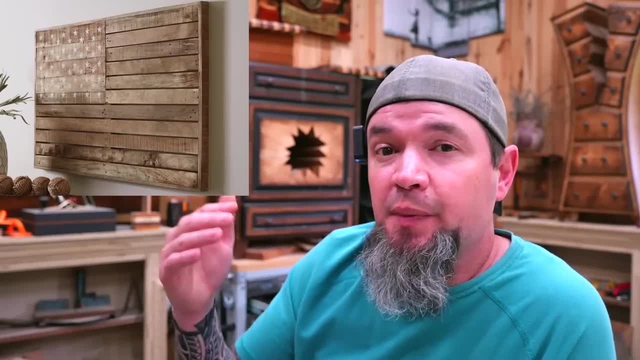 be the same as you did for the bottom. I'm going to take a 48 inch strip and I'm going to cut the extra strip for the bottom. I'm going to cut it up to the center And I'm going to cut it. 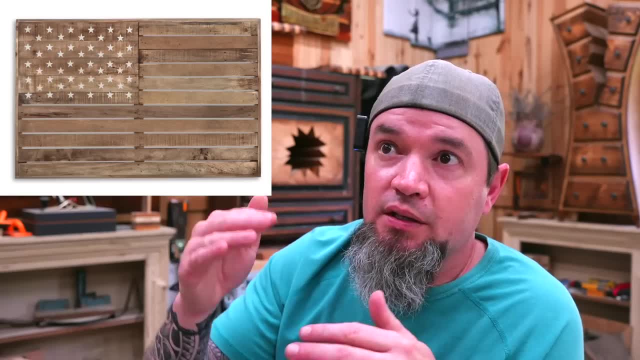 down to the top. Okay, the stars panel. Whenever I say panel, that's all that they have done is taken those 24 inch pieces and stack them flush on the left hand side all the way to the top As far as the star pattern. 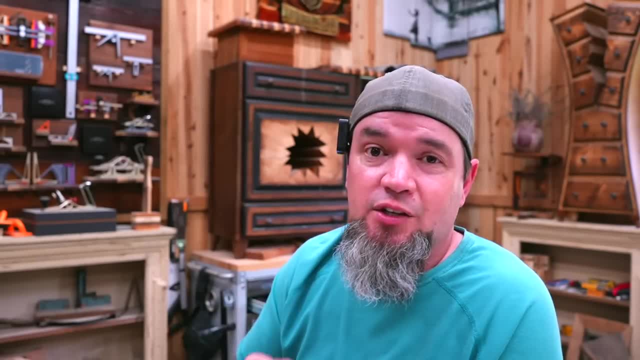 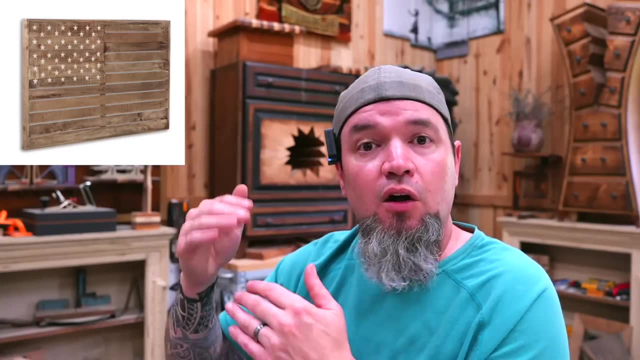 itself, that is paint. So that's all that they have done is taken a stencil Again. you can pick these up off of Amazon for dirt cheap and about any size that you would like, And most likely before they nailed them to this, they had all of those boards off to the side, put the stencil on. 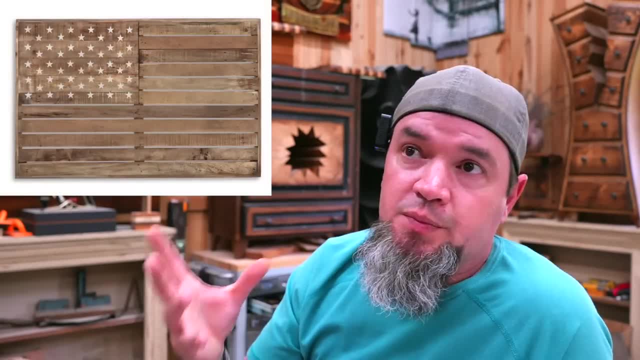 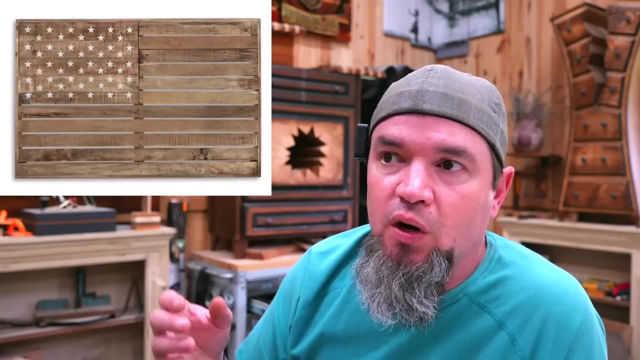 add some white spray paint to it and then attach those boards to their flag. So at this point you have all the front made and the back, And now that's all we need to do is put on our side border. And really the only reason they put this side border on is to kind of hide the underboards. 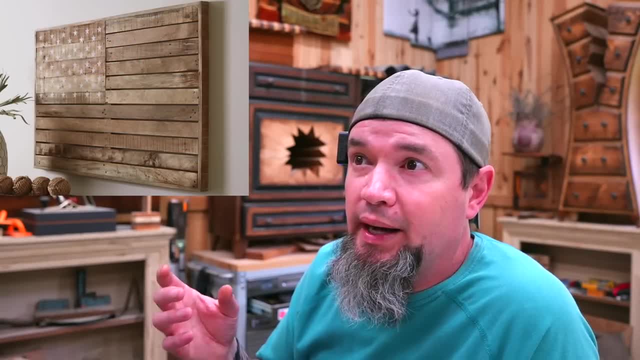 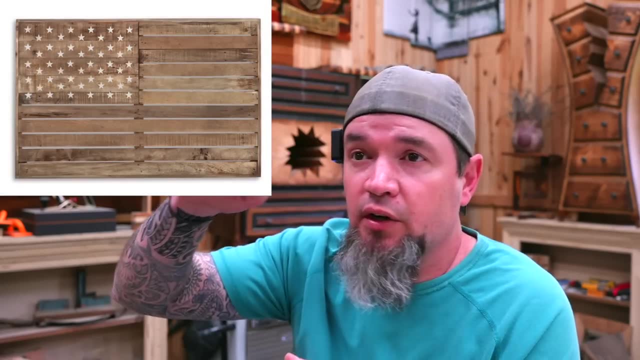 So to me it looks like the border is just about an inch, maybe an inch and a half wide. They did not even miter the corners. These are just butt joints. They're going for that rustic, primitive look. So now you would just add your border covering all those edges that we're talking. 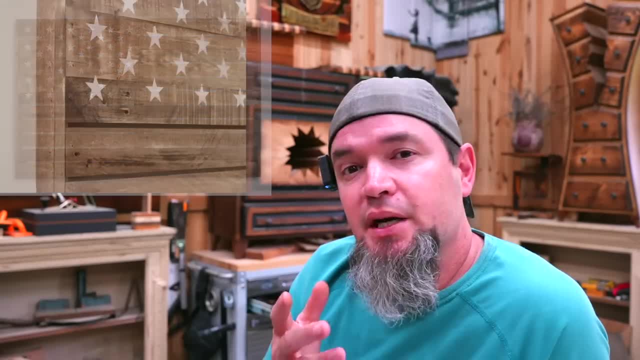 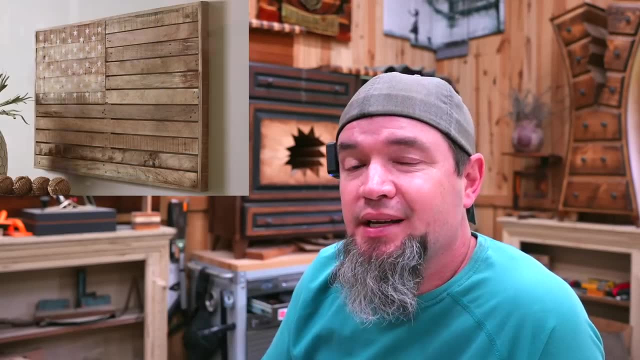 about and then just attach this border using brad nails and wood glue And make sure that you get a nail or two into each one of these horizontal strips. Again, they went 150 bucks for this. I'd put these out there at about a hundred bucks a piece and you don't even have to put a finish on. 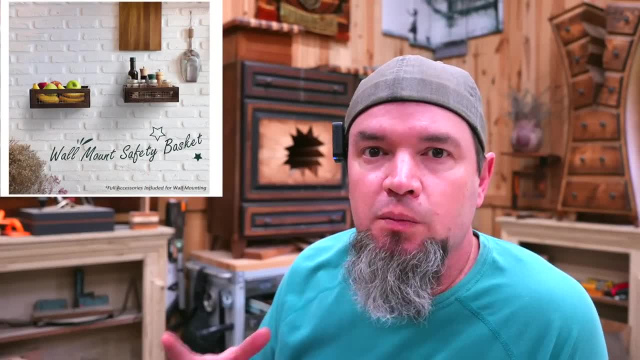 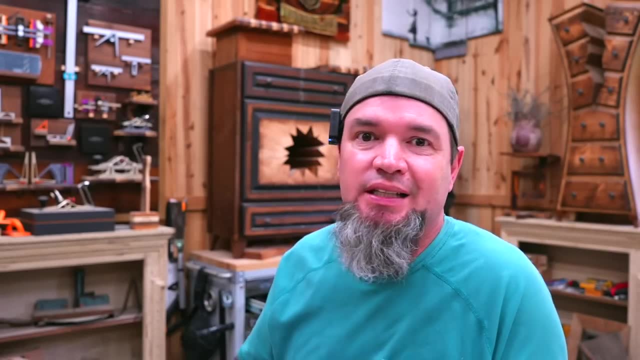 it Okay. So this next one. they are marketing these as mountable boxes and they're super cool And, yes, everyone loves boxes And I cover a lot of different things on crates and boxes. It's just because it's an evergreen type of an item. You can sell it year round and it always stays. 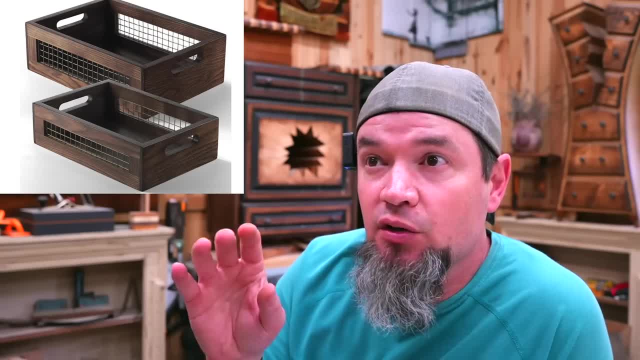 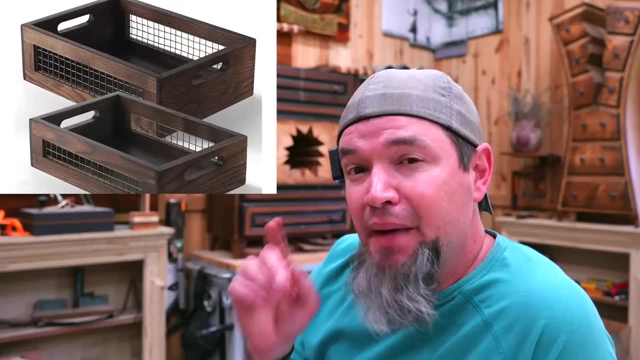 in style. But this design I have not seen before. They've actually integrated hardware cloth into the edges, And then you have your typical ends. That makes it different, That makes it marketable And that is what is making these things sell. So let's go ahead and discuss these ends And 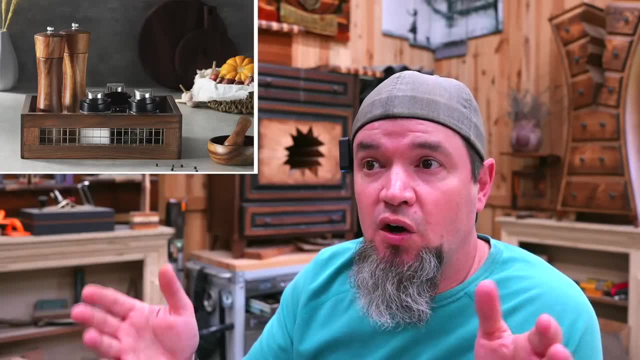 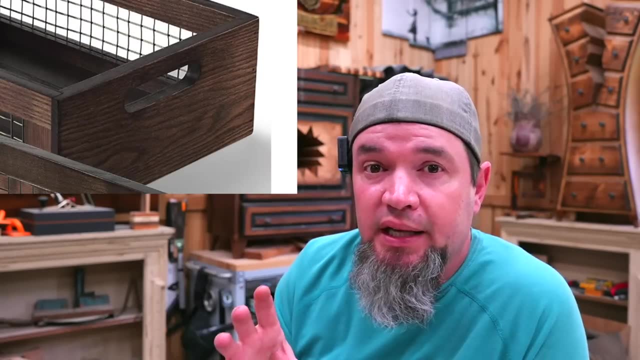 I'm going to show you what I've done before. Solid wood is about four inches wide and about eight inches long, And then that's all that they have done is cut a handle into it. So to cut this handle in, I would measure in a couple of inches from each side, measure about an inch down from. 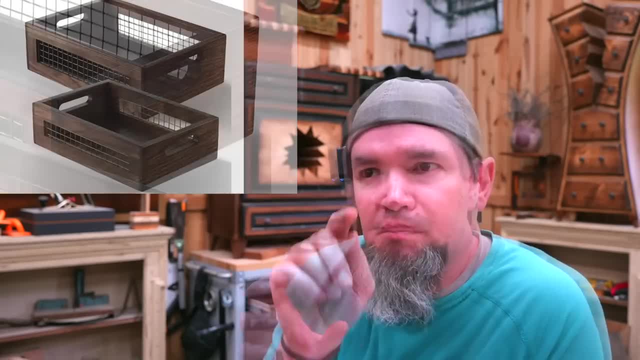 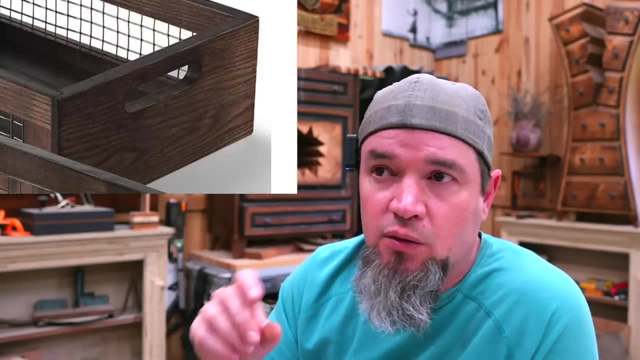 the top and that will leave you with four inches of handle. So I've centered that in marked the edges where you're going to cut that out, The two outside edges, I would use a spade bit, whatever thickness that you would like this handle. Let's say, if you want an inch opening, then just use an. 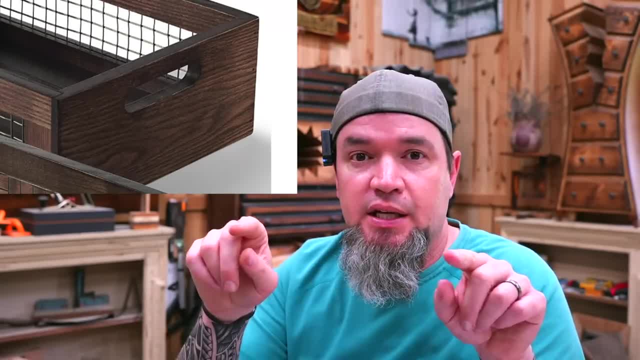 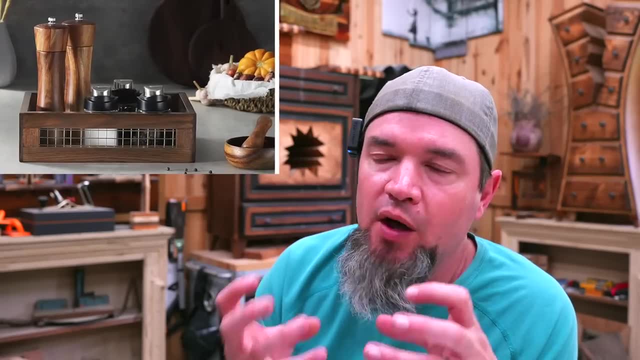 inch spade, bit forstner, bit whatever it's you would like on each end, And then take a jigsaw and connect those two holes, removing that center part. Then you would just repeat that for the other side. So now let's get down to how they actually put this hardware cloth in there. So 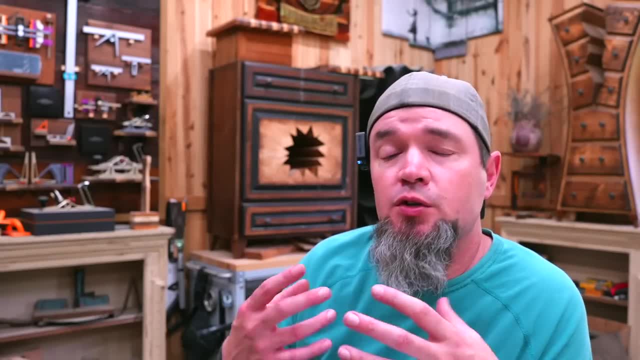 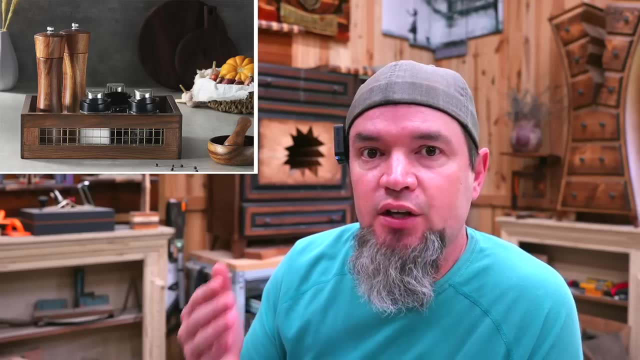 first of all, you just need to decide what size hardware cloth that you want to use. You can pretty much pick it up at any type of hardware store, but the squares that make this up are different sizes And if you look at this, it looks like that the hardware cloth is actually made. 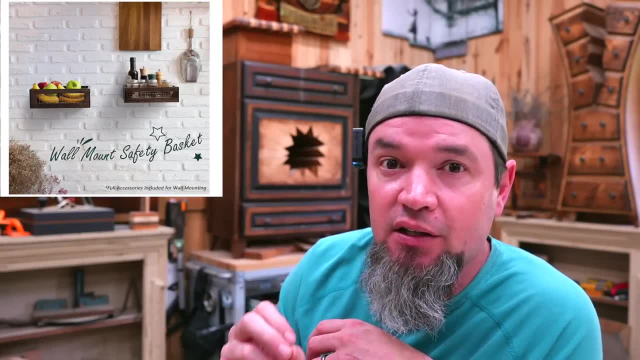 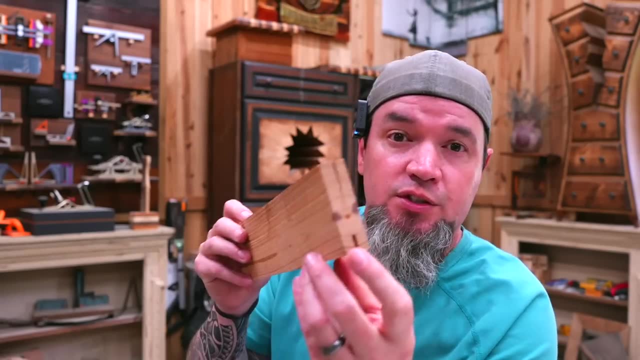 into the wood itself, And what they did to get that nice, clean look is super simple. You need to make a groove in your material, And this is simple to do, So all that you have to do is set your table saw to where it is in the center of the board. that. 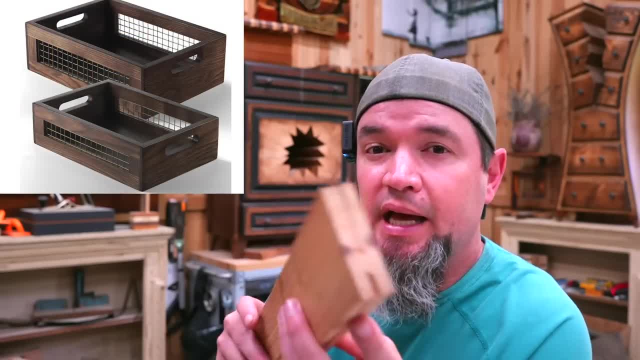 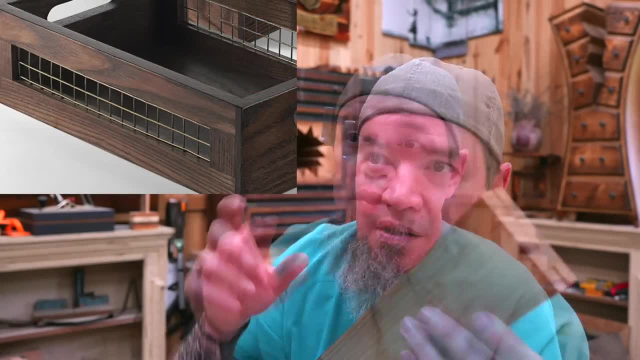 you're cutting and then set your depth. That's all that it will take, for this design is about a quarter of an inch of depth, because each one of these strips around the hardware cloth, since the total height is four inches, those are only about inch wide strips. So instead of trying to cut your 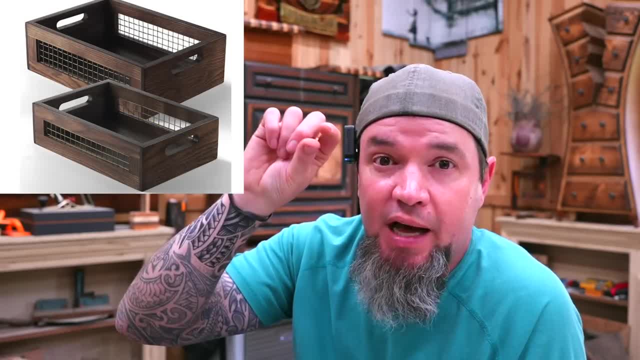 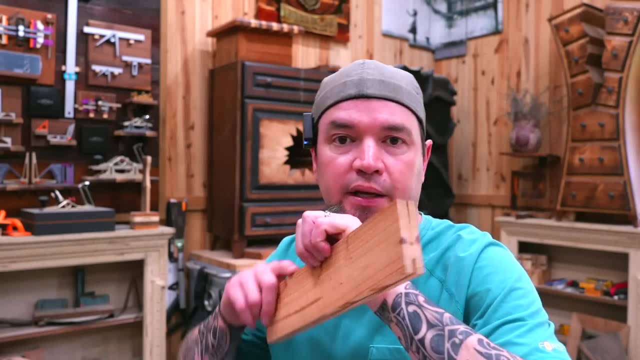 two long pieces, the top and the bottom, and then your two side pieces into little pieces and then run them through your table saw. just cut one long strip from this groove, which is the thickness of your table saw blade, through the center of the center of the table saw blade and then cut the. 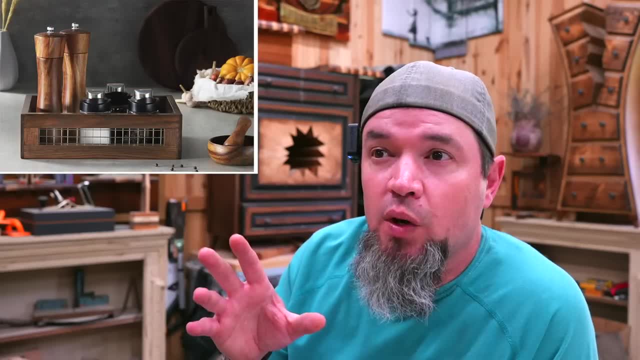 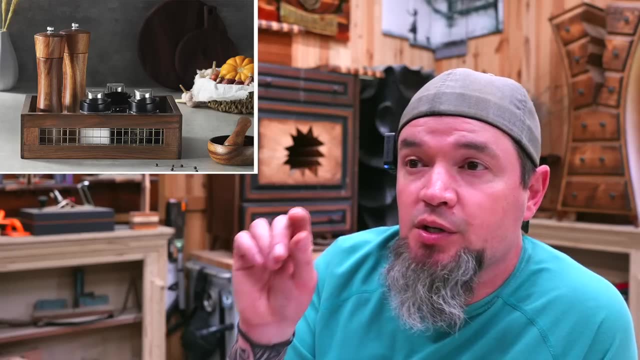 entire board, And then you can cut your parts to size. So if this box is 12 inches long and the handle parts are on the outside of this, let's say that you're using three quarters of an inch material. the horizontal side strips are going to be 10 and a half inches long each, And then your 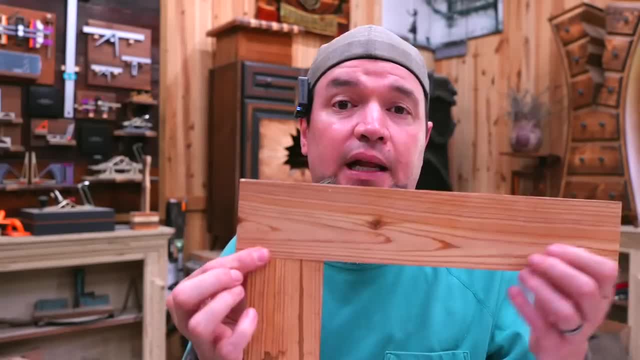 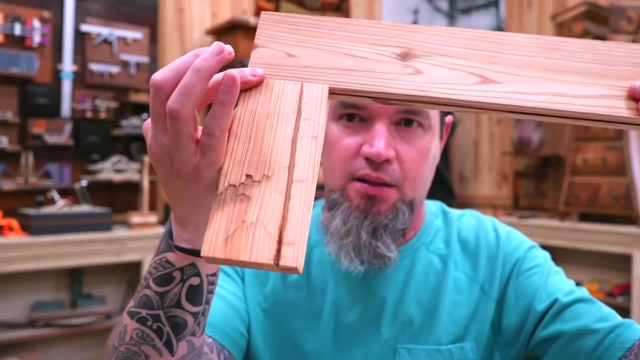 two small vertical strips are only going to be two inches long each, And I know my example is wider boards. but whenever you set these on top of each other- and again these are just butt joints- it's going to sit like this, but the inside will look like that. That is where your hardware cloth. 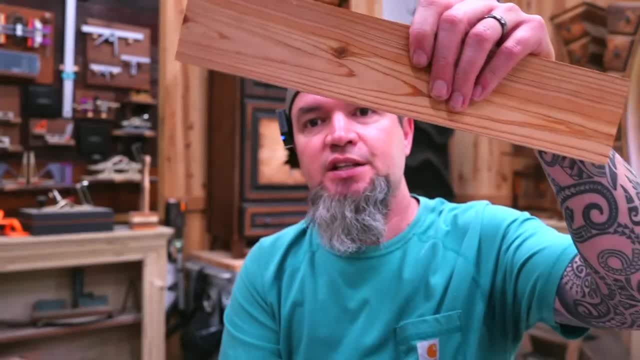 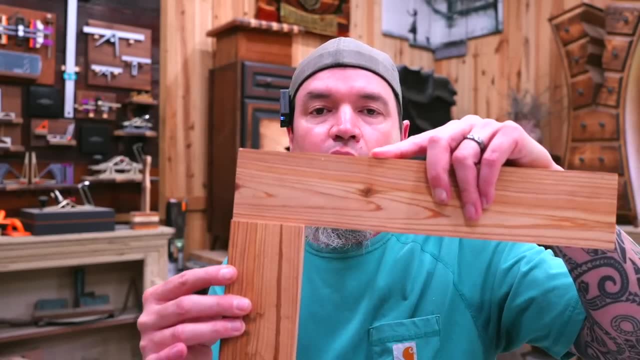 is going to go. So you cut your hardware cloth to size, go ahead and insert it in between your two long boards. Then you would just slide your end board over on each side, locking in that hardware cloth right into those little grooves that you've made. And that's all that they have done to lock these in. 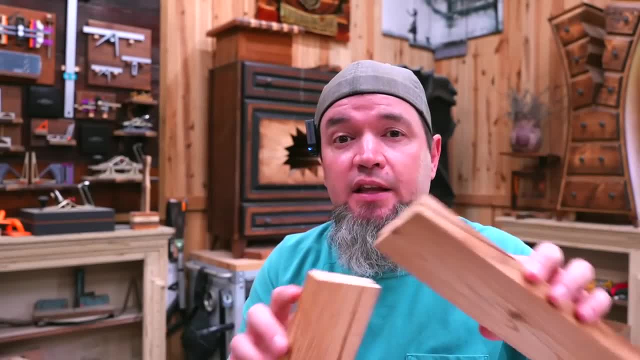 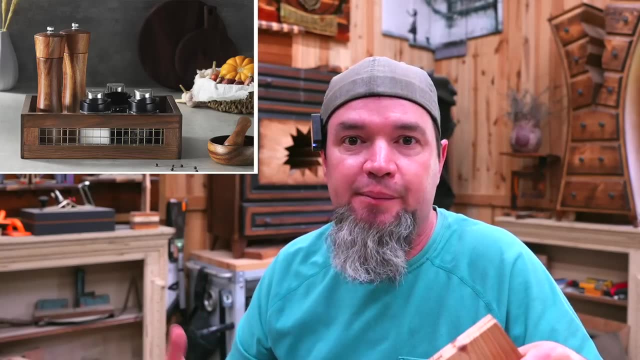 the place, because these strips are only an inch wide each. They fastened this together with brad nails and wood glue. That's all that there is to the side panels, which is the main part of this thing. So you have two end pieces and you have two side panels made- The side panel, if you look at. 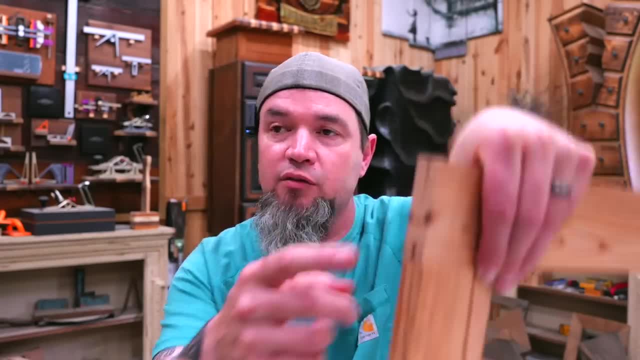 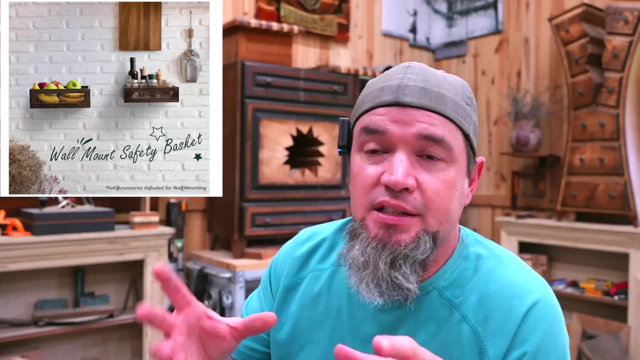 the edge will have this little cutout, But no one will ever see that, because of the design of this box, the handle boards or the end boards will go over that part, hiding all of that. And that's all that they have done is put. 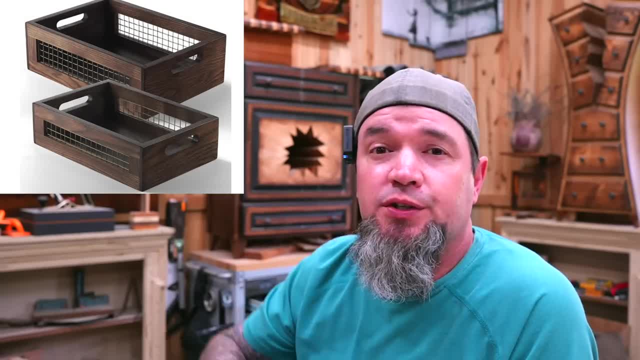 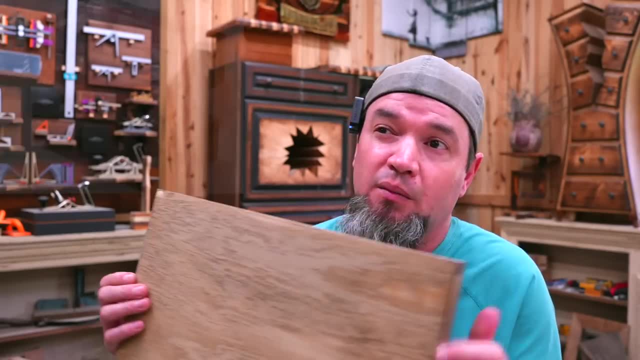 that, together with some wood glue and some brad nails. As far as the bottom goes, you can use whatever material that you would like to inset that, throw in some brad nails, or you can take some quarter inch plywood and nail it to the bottom like they did. So if that came across as 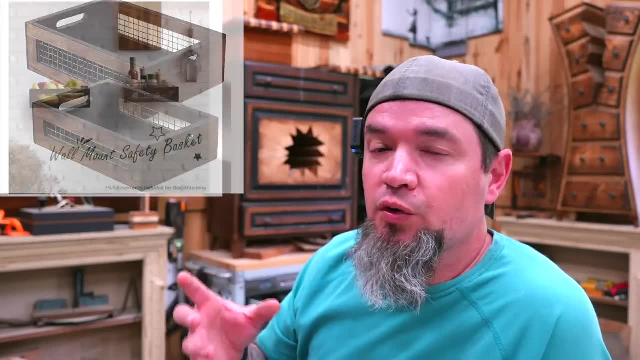 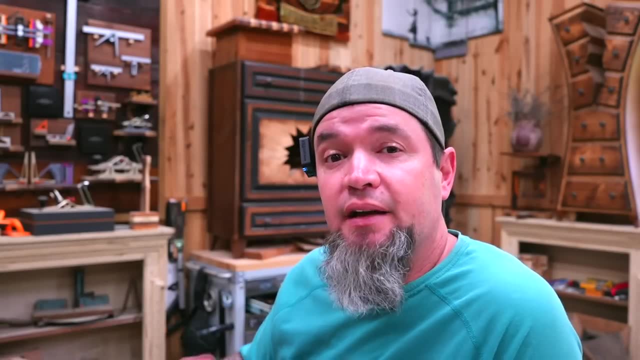 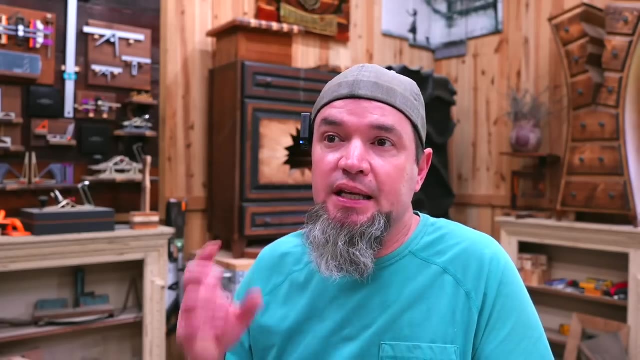 sounding difficult. I promise you that it is not, And when you're done, you're going to have a super cool, unique crate basket- whatever you would like to call it- And they will sell a lot of them. So, if you have one at home, let me show you a couple of things that I've been seeing on almost 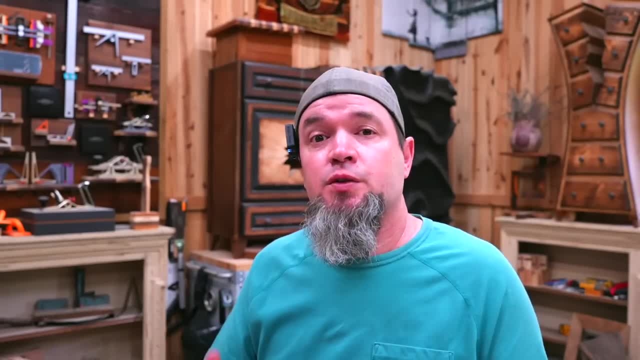 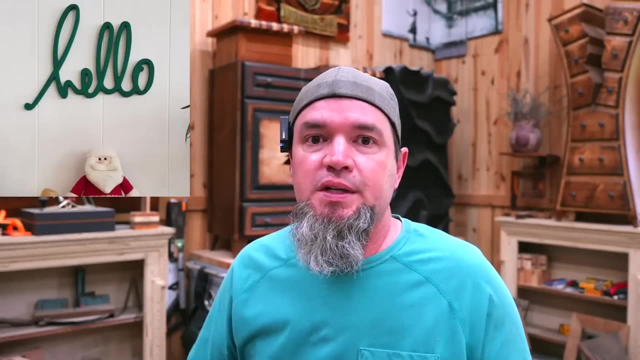 every site. So I've never been comfortable with lasers because I've never used them. But after a few months of using my Thunder Laser, it's pretty cool. So I'm going to head over there and we're going to talk about this first one. So this first one is going to be basic signs. okay, Except you're. 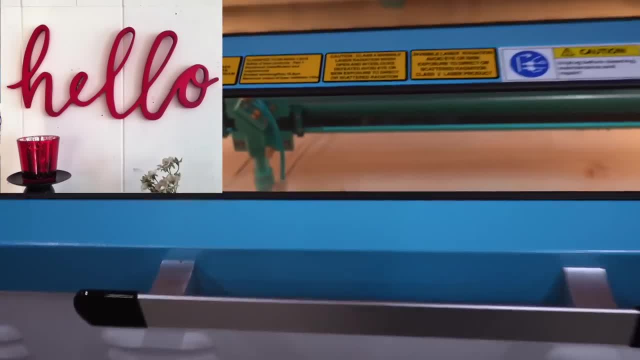 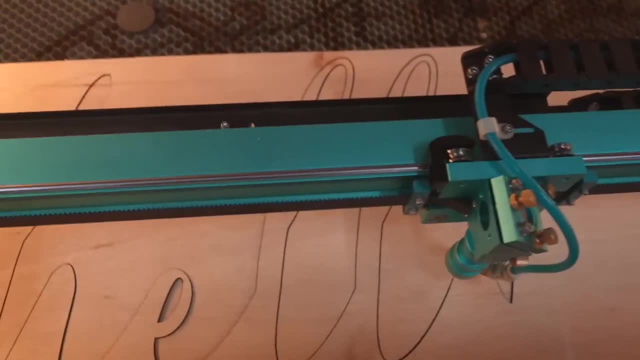 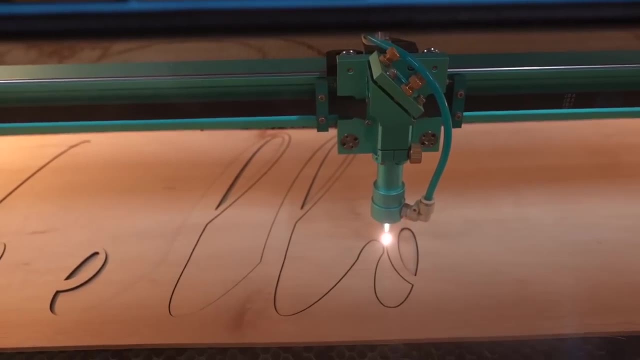 like this. This is just hello, But it is a 16 by 15 cutout. I've seen different variations of just this one word on several sites. On all of the different sites that I have found these. they were wanting between $50 and $75 a piece. And this next style is super cool. I've seen it everywhere. 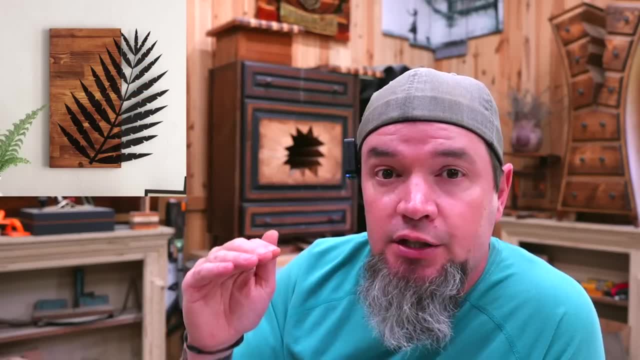 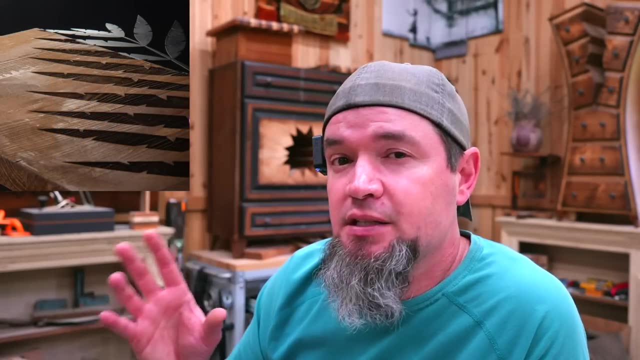 and it's always on people's bestseller list. I've used a laser to etch the wooden parts of these designs. For everything that hangs over the wood, it's actually metal. What if we use our laser cutter to cut this out of a thin piece of plywood and just paint it a color to match what we have? 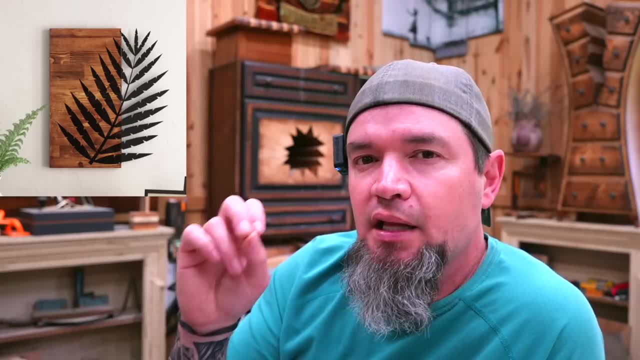 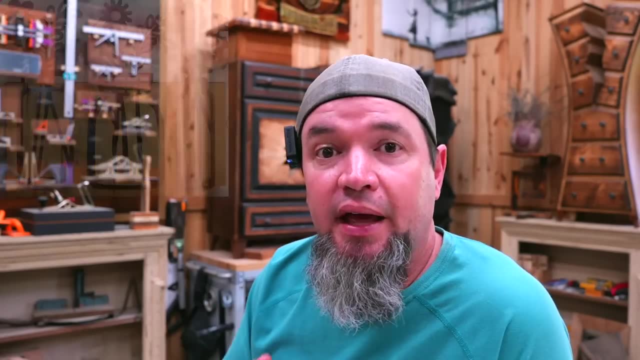 burnt. Attach it to the sides and you have an awesome piece of art that's selling for upwards of $75 a piece everywhere that I've seen them. So that's just a couple of ideas that I've ran across and thought about you guys out there that had laser cutters. Well, thank you guys, so much. 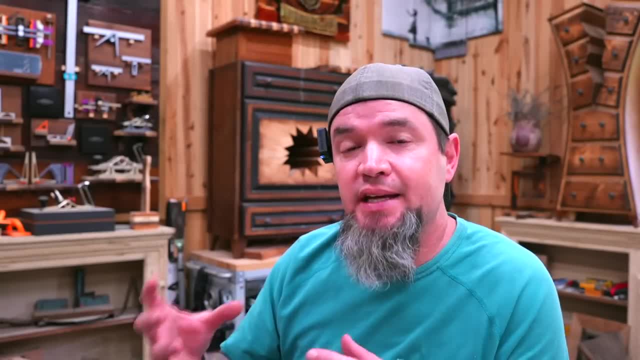 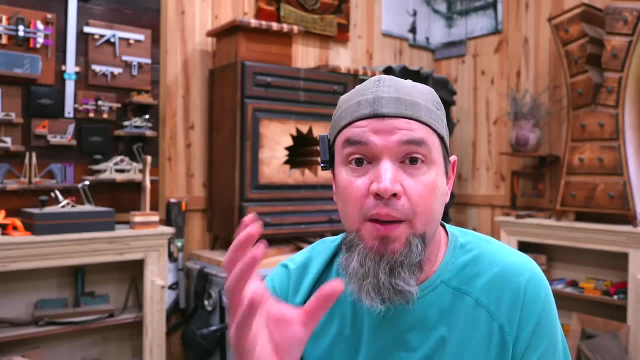 for watching. I hope that you have enjoyed today's video and you were able to take something from this. apply it to an idea that you have and run with it. Practice breaking it down in your head on how it was built. Go home and replicate that If it doesn't work out the first time. 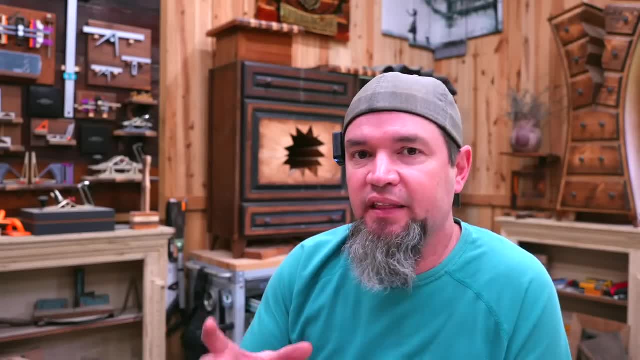 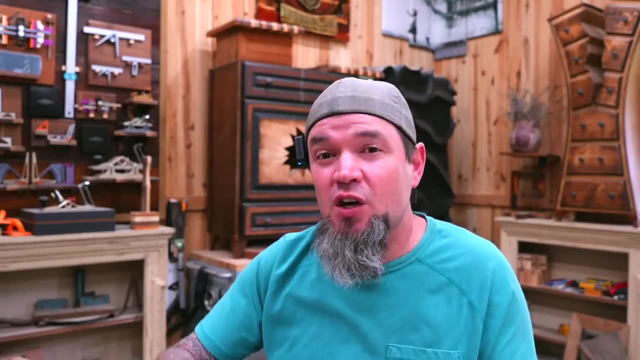 keep practicing. That's how we do this and that's how we learn. And then, whenever you come across a project that integrates several of these different things that we've broken down, it'll be a piece of pie. So, as always, go out there, be creative, think divergently.